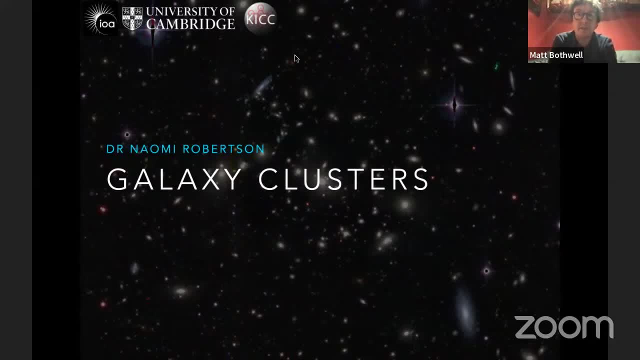 Robinson, who is a postdoc here in Cambridge, and she's going to be telling us all about clusters of galaxies. Over to you, Naomi. Okay, thanks, Matt. So yeah, it's great to be here to chat with you this evening about one of the areas of research that I work on here in Cambridge. So when we look out into the 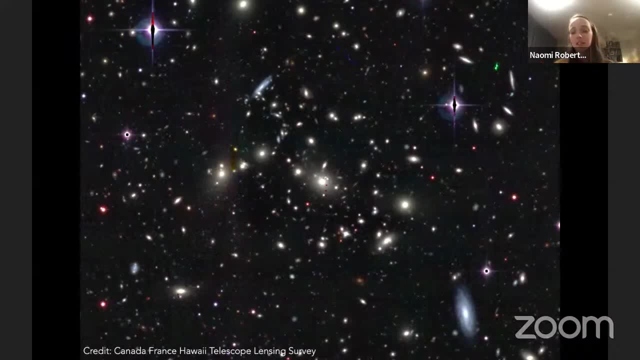 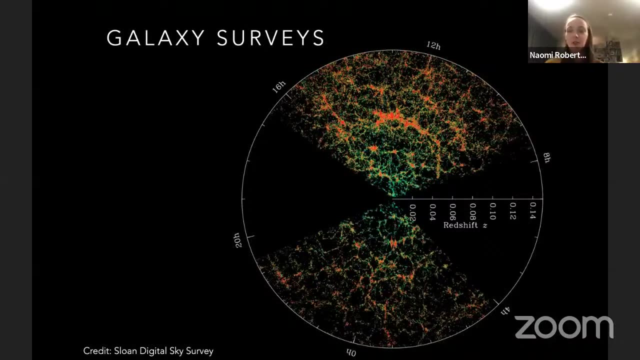 universe, we see that galaxies aren't randomly distributed across the sky. Instead, galaxy surveys like the one displayed here have shown us that galaxies are in fact clumped together, with some parts of the sky appearing to be denser than other parts. So this is data from 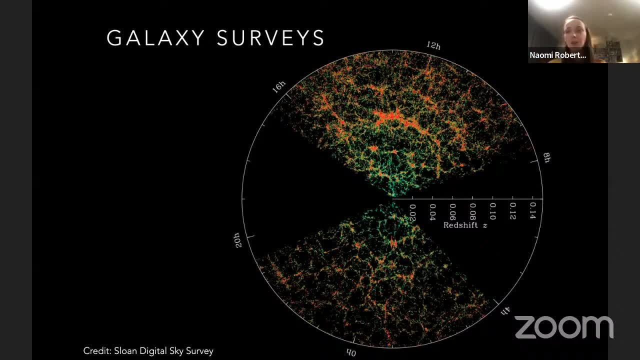 the Sloan Digital Sky Survey, which really accurately maps out where galaxies are in the nearby universe and the pattern that we see here in the plot. we can see that they structure really clearly in the galaxies. So on this map we are located here at the centre of the circle and as you move out away from the centre we are looking further and 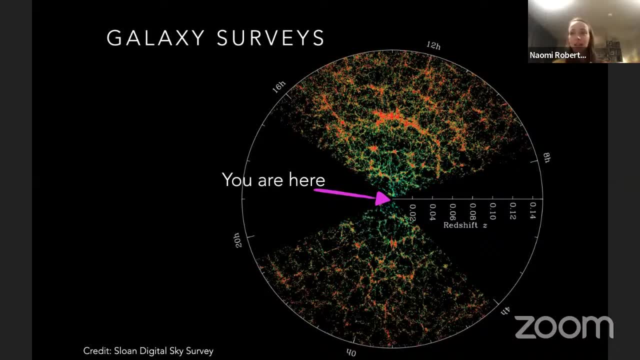 further away. So, since light takes a certain amount of time to travel, as we look further away from us, we are looking further back in time, So this one has some of the largest. So what we're actually seeing is the universe when it's younger, as we look further and further away. 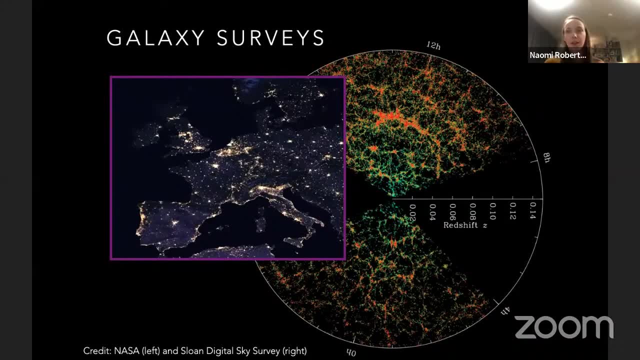 So if we look at this image of Europe at night, we can see that where most people live are where most people live just by looking at where the lights are, And so the lights show us where all the towns and cities are, So we can see London and Paris and Madrid. 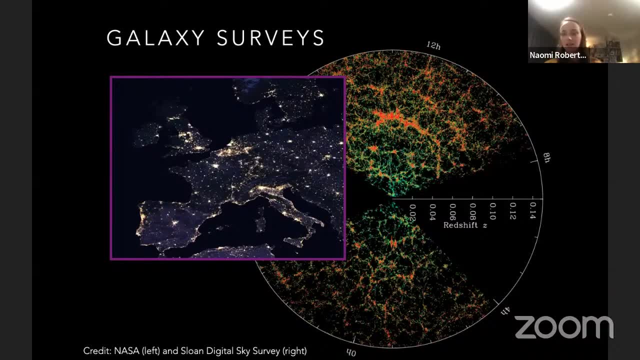 And, similarly, this is what this galaxy map is telling us. So the brightly coloured parts of the galaxy map which you can see here, they tell us where the galaxies live, And the red parts are where there's lots and lots of galaxies. 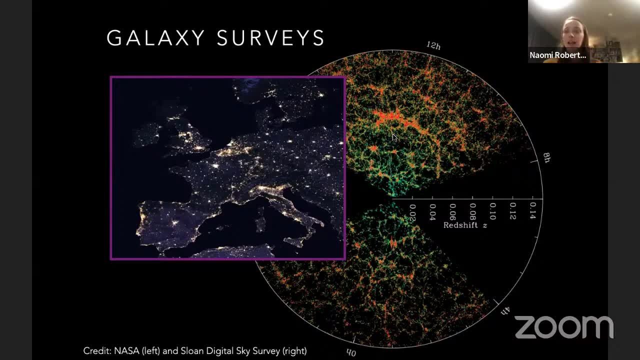 The green parts are where there's fewer galaxies, And these darker regions are where there's almost no galaxies at all, And so we don't just see the structure in the galaxies, but we also see it in the dust and gas that we see in the universe. 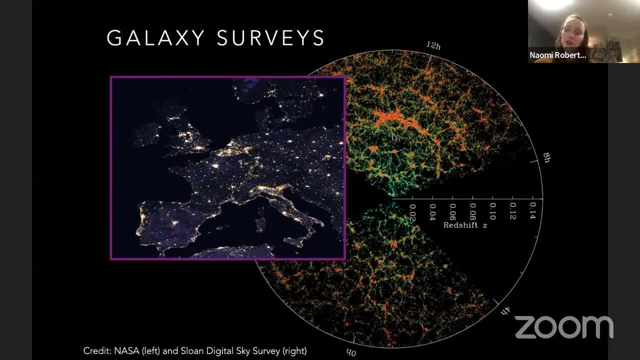 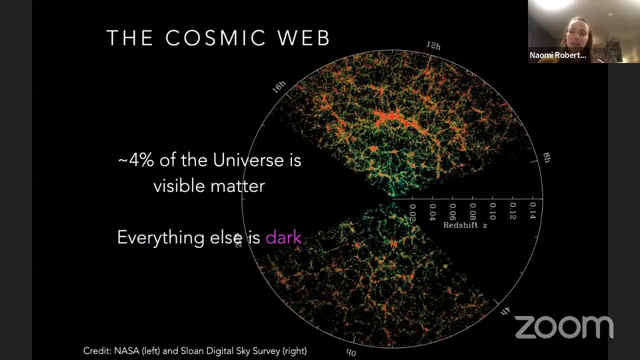 And astronomers have shown that. So I've coined a term for this structure that we see called the cosmic web. So these observations of galaxies and dust and gas are what we refer to as visible matter or baryons, And this is what we can make measurements of with conventional telescopes. 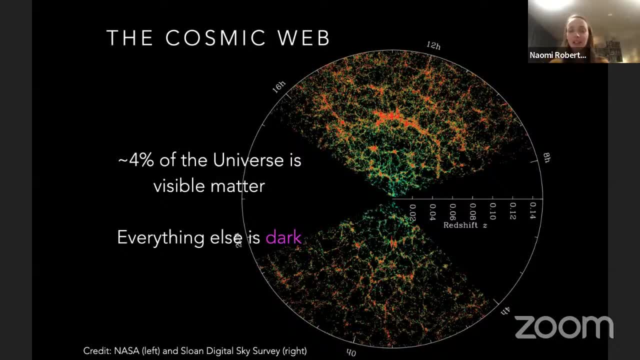 Staggeringly, the visible part of our universe only accounts for a mere 4% of it, So that's a tiny, tiny amount. Everything else is invisible And we refer to this as visible matter, And this mysterious part of our universe is dark. 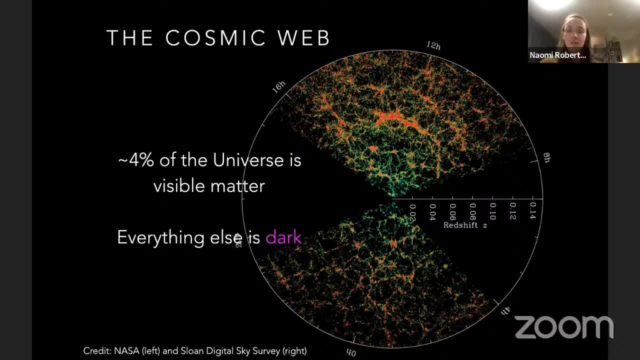 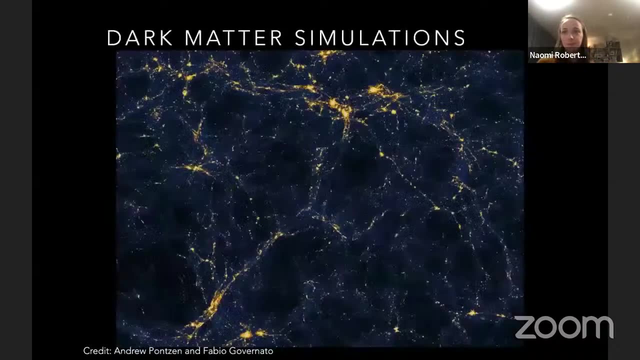 And this has been one of the main challenges for modern cosmology to figure out. So we know that this part of this part of the dark universe called dark matter and the gravitational pull of dark matter holds stuff together at small scales, And so scientists have performed simulations of this dark matter based on the idea that it only feels the force of gravity. 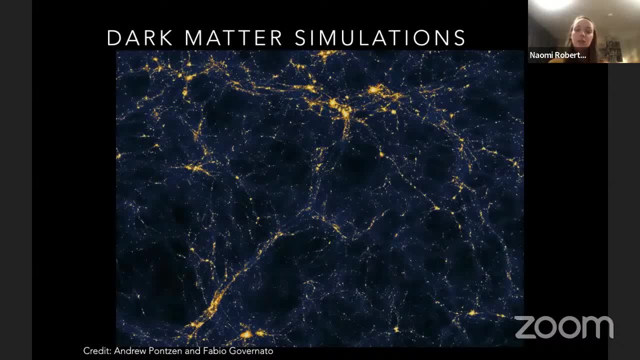 And what they have found is that dark matter also forms this web-like structure And this is what is shown here. So this is a simulation of dark matter, And the brighter parts of this image show where there's a dense region of dark matter. 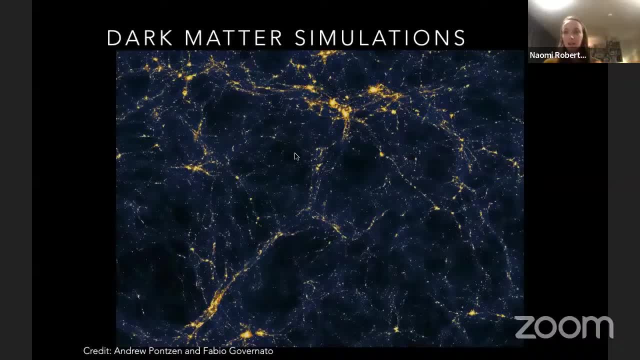 And the darker parts are where we see very little dark matter. So you can see these same strands of material that we saw when we looked at the map of where the galaxies are, And so this cosmic web isn't just in the galaxies and the gas. 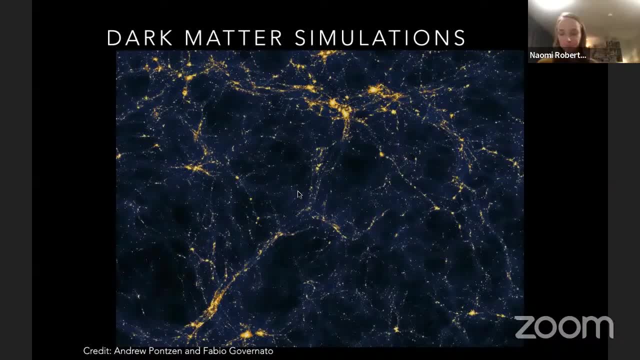 But it's also in dark matter itself. So, putting these two findings together, we now believe that dark matter forms the skeleton of the cosmic web And that galaxies follow the pattern that the dark matter makes. So where we see lots of galaxies, we also expect to find lots of dark matter. 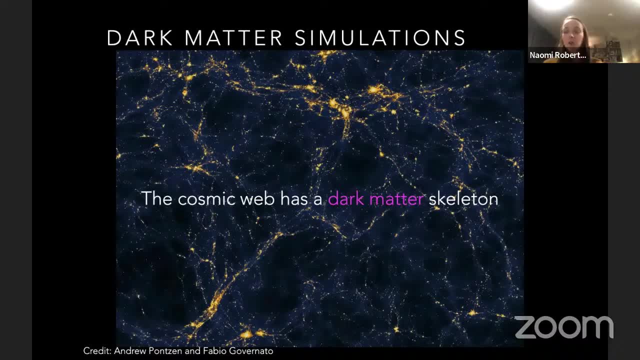 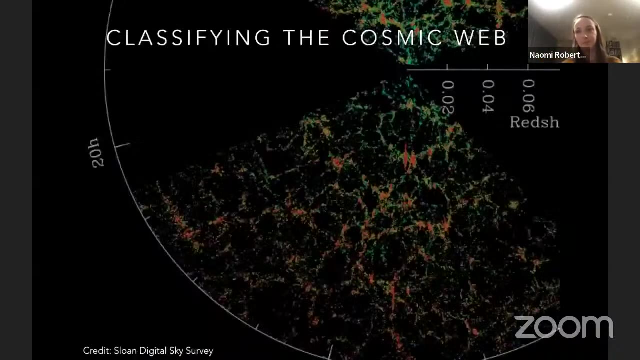 And where there are very few galaxies, there will also be less dark matter. So this is just like how the light on that image looks. The light on that image of Europe at night told us where people live. The galaxies here trace out where we can find the dark matter. 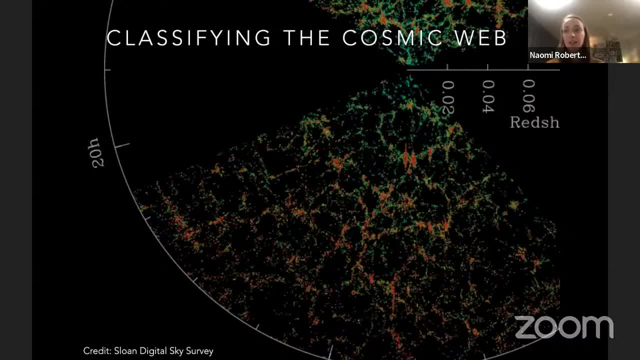 And so if we go back to our image of our galaxy survey- and here I've just zoomed into a small portion of it- we can see that this cosmic web structure is a bit clearer. And what we do is we classify the cosmic web into categories. 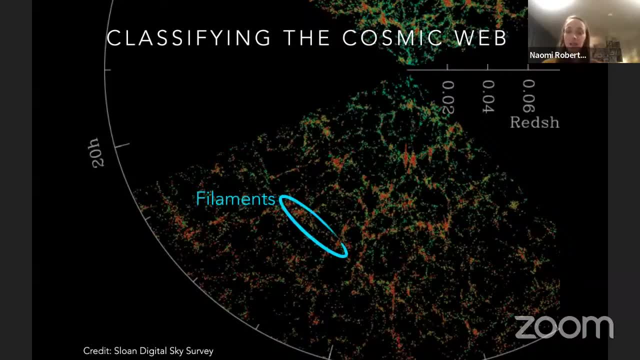 So what we refer to as the strands of galaxies, we call filaments- and this is what I've highlighted here in blue- And these form a huge component of our cosmic web, And we find that these filaments can cover huge different ranges of lengths across the sky. 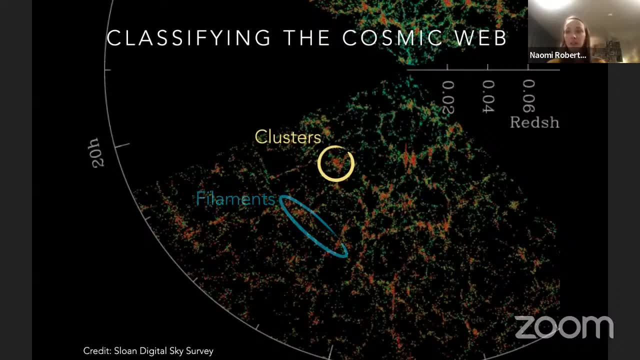 Then, where we see these filaments intersect with each other, we get even denser regions, And this is where we find clusters of galaxies And then, in the spaces between the filaments and the clusters, what we refer to as voids. these voids are very large regions and they contain very few galaxies and are really the emptiest parts of our universe. 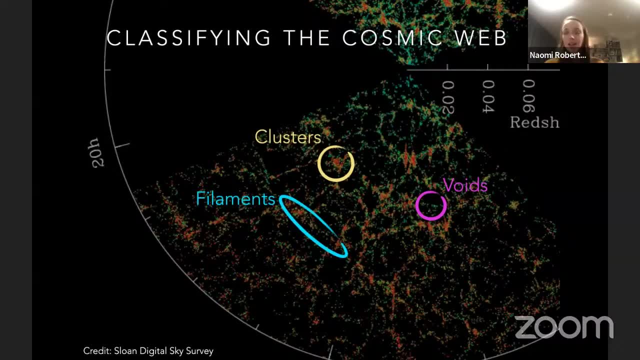 So we divide up our web into these three components. And galaxy clusters are really like the cities of our universe. They're very densely populated with galaxies, The filaments are a bit more suburban and the voids are like being out in the countryside. 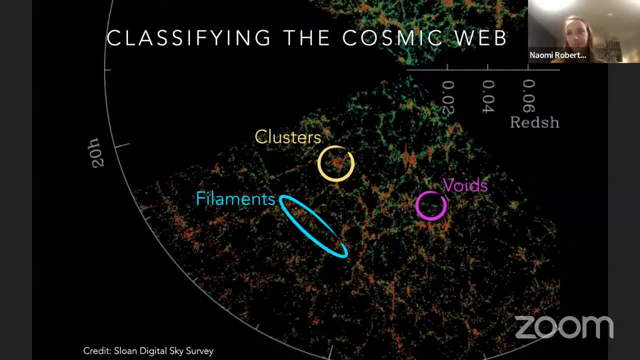 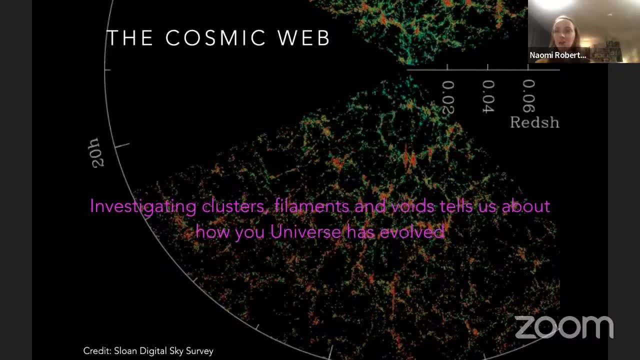 There's not much there, Not very populated at all. So from a cosmologist's point of view, observations of the cosmic web is really key to understanding how the universe formed and evolved and to become what we see today, Given that the cosmic web traces the dark matter in the universe. 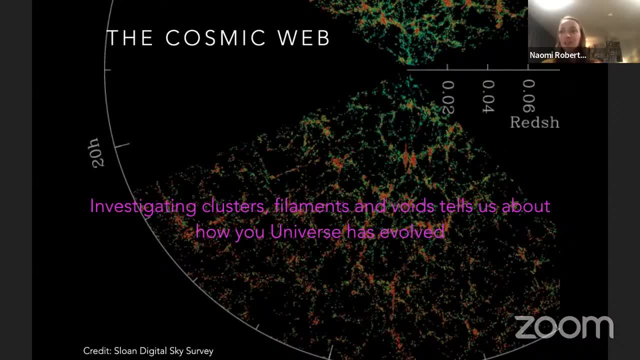 we can use the cosmic web to try and understand the dark matter itself, And what we do in practice is we take our best model for how we think the universe formed and then test that against the measurements that we make to see how well it can explain what we've observed with our telescope. 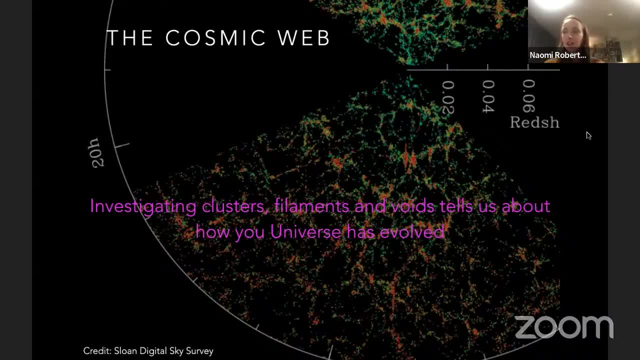 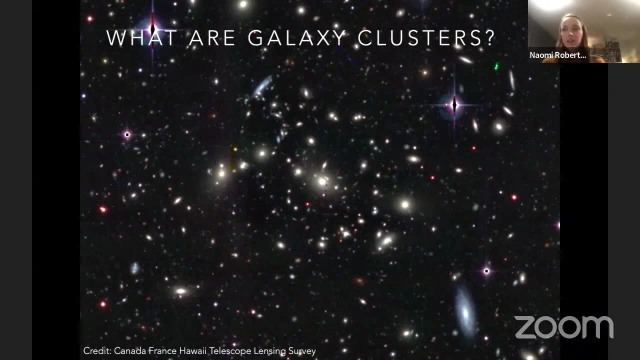 So the densest part of our cosmic web is particularly interesting, and it's what I work on myself, And so for the rest of this talk is going to be focused on galaxy clusters. So the first recorded observations of galaxy clusters are from the 1700s. 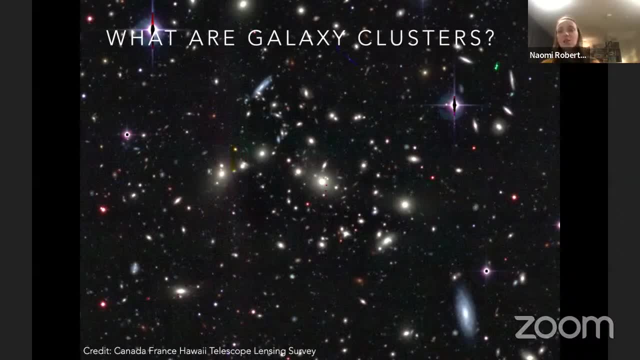 and they were made by Charles Messier. He published a catalogue of astronomical objects called nebulae, which later became known as Messier objects, And he didn't know that some of these nebulae were in fact clusters, as what he was originally interested in finding was comets. 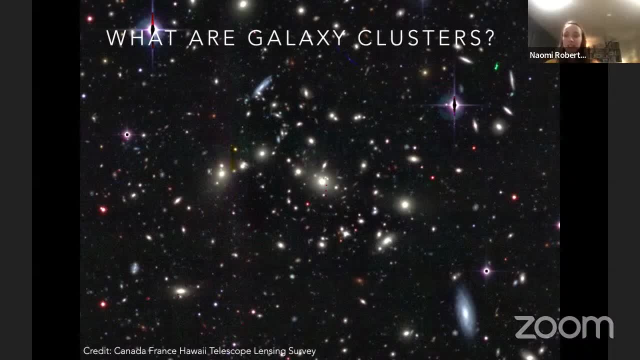 which only appear very briefly in the sky. So, to save time, in the grand scheme of things, what he was doing was noting down any object that he thought looked a bit fuzzy, like a comet does, but that was always there and it wasn't this transient object. 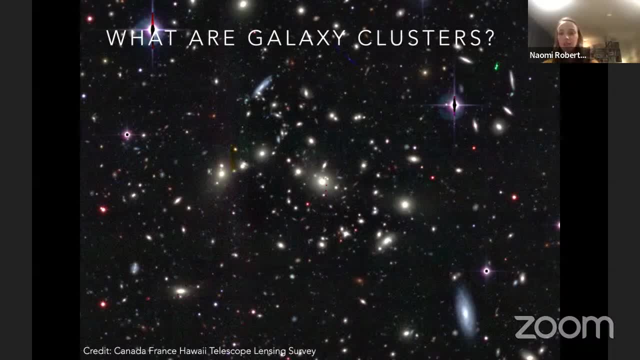 So this ranged from star clusters, which are in our own galaxies, to actual galaxies which are a bit further away, or also clusters of galaxies which looked fuzzy but were even further away again. So, therefore, it was only once that we had the ability to measure distances to these objects. 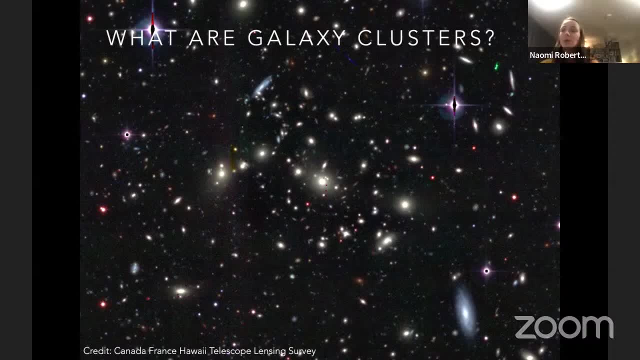 which happened in the early 20th century, that we were able to find out what these objects actually were, And this is when we identified that some of them were in fact, clusters. In the 1950s, there was a more organised effort to catalogue these clusters. 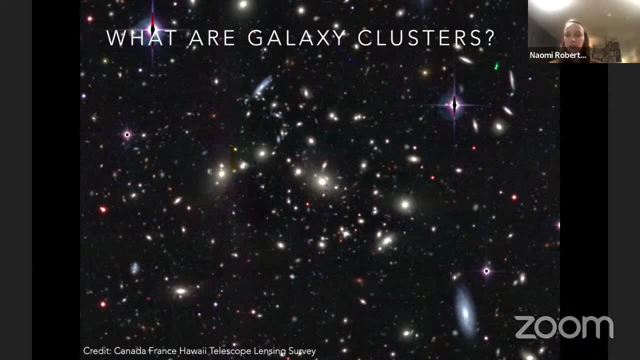 and that was made by astronomer George Abel, and a lot of the clusters are named after him. So these galaxy clusters, they're exactly what the name suggests: They're a large group of galaxies. Typically, clusters contain hundreds to thousands of galaxies and they're bound together by gravity. 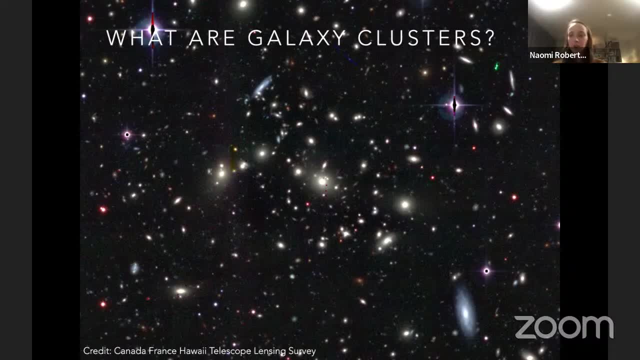 They are, in fact, some of the largest gravitationally bound structures that exist in the universe. We used to think that they were the largest, but then we found superclusters, which are even bigger again, and they're clusters of clusters. So, but to be honest, they're not. 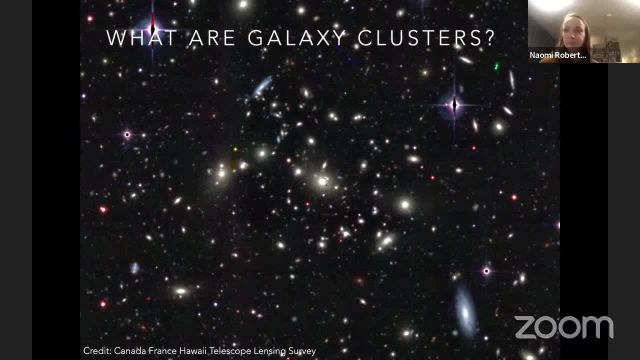 Today we're just going to stick to clusters of galaxies. So when we look at an image of these clusters, we tend to find that the biggest and brightest galaxy in the cluster tends to be located at the centre, which I've highlighted here for this galaxy cluster. 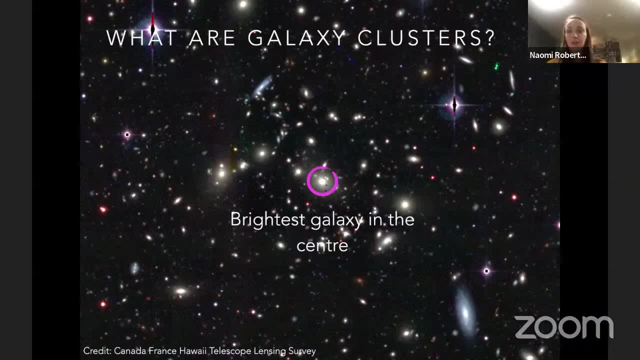 Then all the other galaxies in that cluster orbit around the centre. So clusters can look quite different and have a variety of properties, and this can depend on how old the cluster is and if it's merged with other galaxies. So let's look at some of the nearby clusters lately. 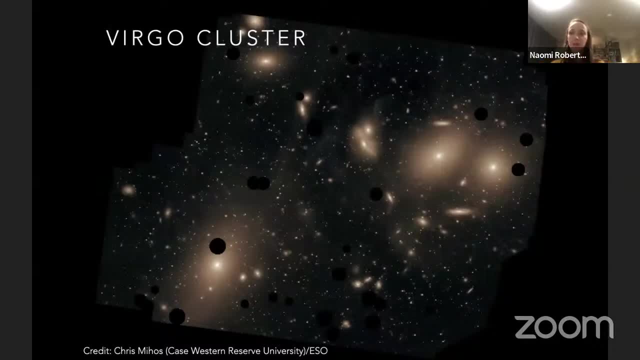 So, for example, this is the Virgo cluster. So the Virgo cluster is the closest massive cluster to our own local group. So this cluster contains over a thousand galaxies, and it's therefore what we refer to as a rich cluster. Now, by rich, I mean that it contains lots of galaxies. 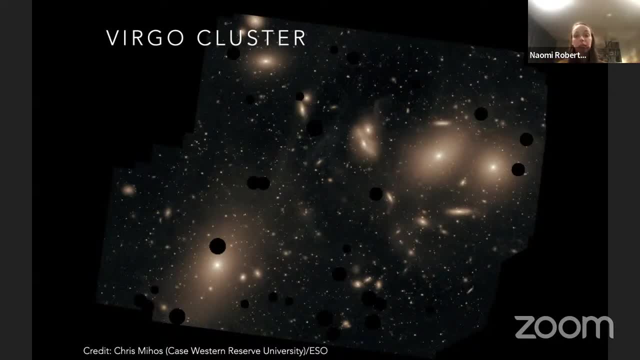 and a poor cluster would mean it contains very much fewer galaxies. So the black circles here on this image are just where there's been foreground stars in front of the cluster that have been cut out, so we can just see the galaxies inside the cluster. 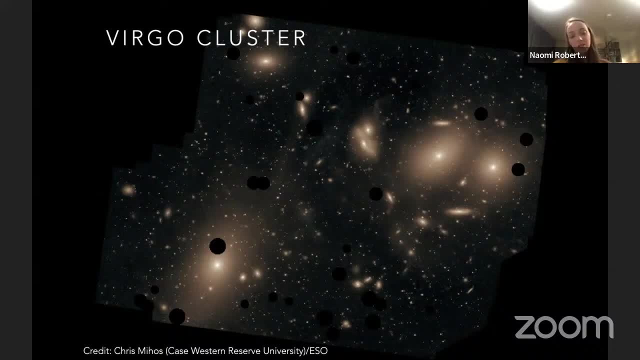 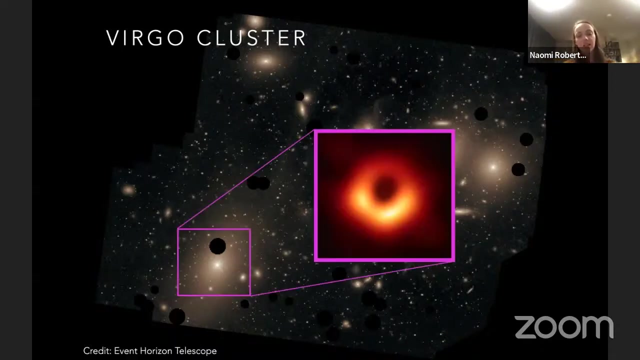 So because this cluster is really close by- it's our nearest neighbour in terms of clusters- it's been studied quite thoroughly and it was actually one of the objects that was first noted down by Charles Messier in his original catalogue. So this galaxy on the left hand side is known as Messier 87. 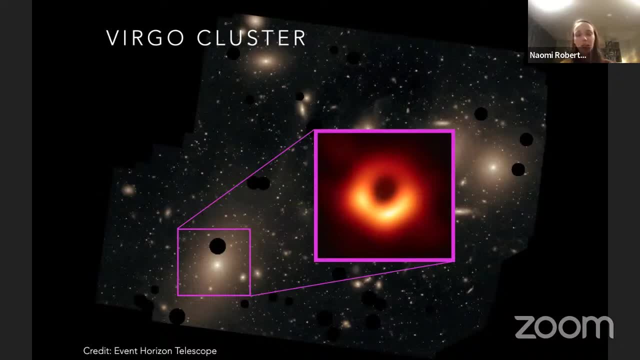 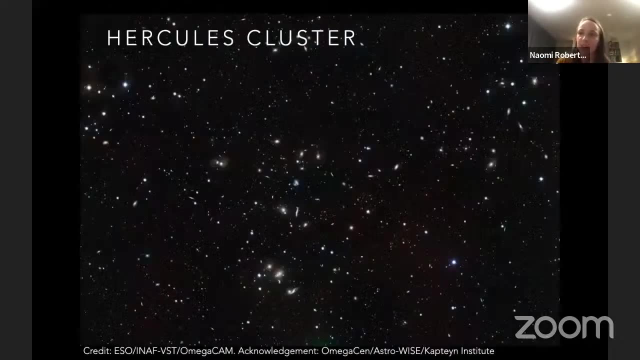 and this galaxy hosts the black hole that had its picture taken by the event horizon a couple of years ago, So I'm sure some of you might have seen that. So another cluster is shown here. This is the Hercules cluster, which is also well known. 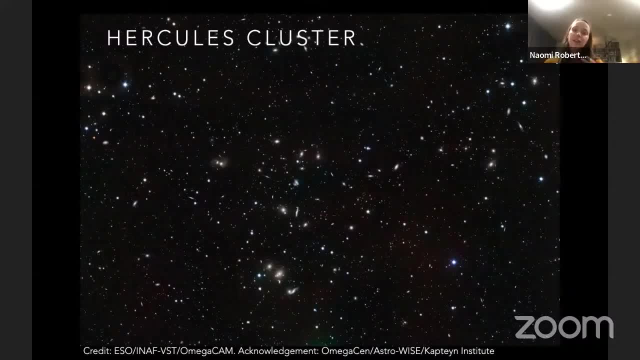 In comparison to the Virgo cluster, though it's quite different. Hercules is poorer and only contains around 200 galaxies. Many of these galaxies are young star-forming spiral galaxies, and there's also lots of galaxies inside this cluster which are interacting with each other. 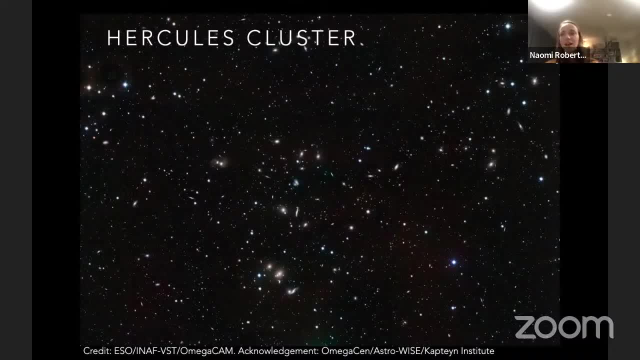 So when we look at this cluster, we see that it doesn't appear to have galaxies very strongly concentrated at the centre or the core of the cluster, compared with other clusters, And so we think it might be a younger cluster and that it's early on in its evolution. 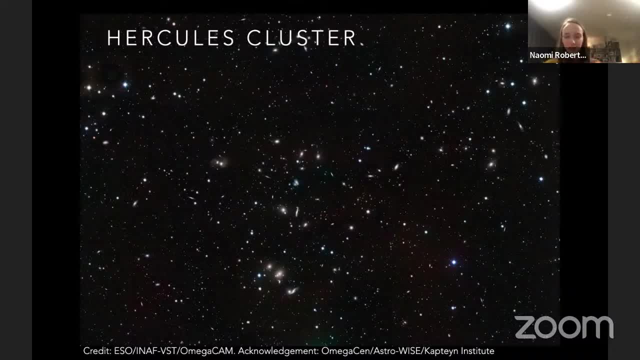 So these are just two of many, many clusters which are incredibly beautiful. Now, in all of these images I'm showing you, we can see the galaxies that they contain by all these little bright spots. These are all galaxies inside the cluster. However, these galaxies only make up around 3% of their mass. 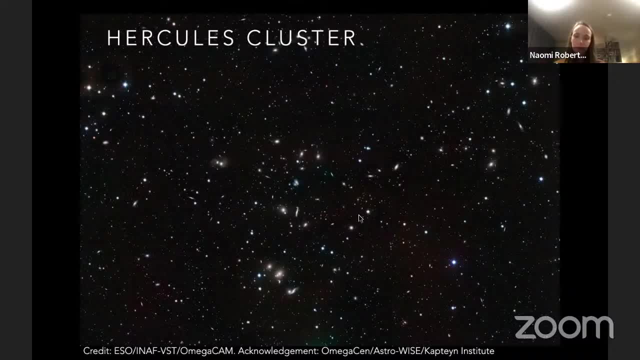 So by mass I mean, if we were to pick this cluster up and put it on our scales, that's how much it would weigh. So what about the other 95%? sorry, 97%. Well, we think about 13% is what we call the intracluster medium. 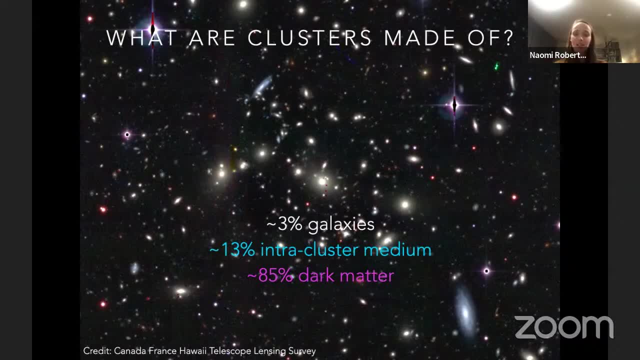 So this is the gas which is inside the cluster. So this gas doesn't belong to any of the individual galaxies itself and it just inhabits the space between the galaxies inside the cluster. Then the remaining 85% is made up of dark matter. 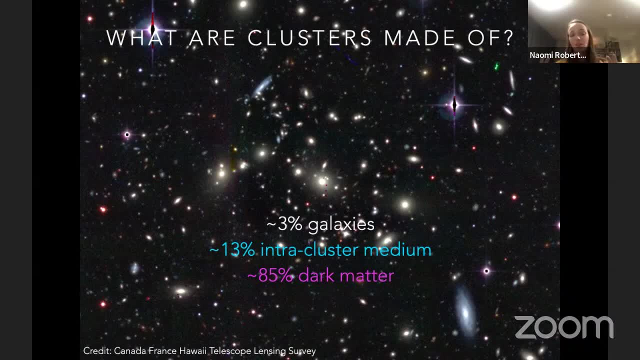 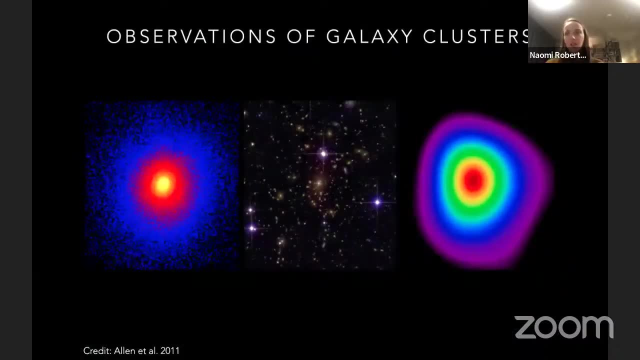 So these clusters are mainly made up of a thing that we can't actually see. So how do we go about finding out what clusters are made of? So, while we can observe clusters at several different wavelengths of light, this has helped us figure out what they are made of. 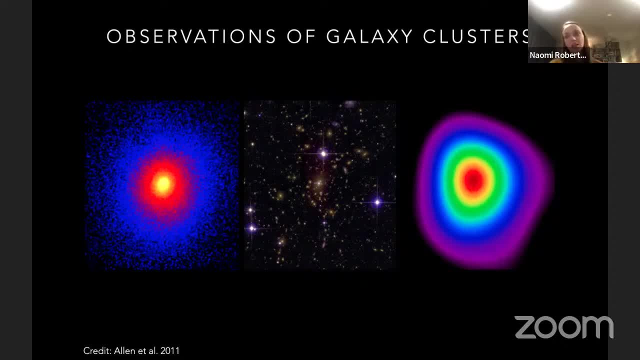 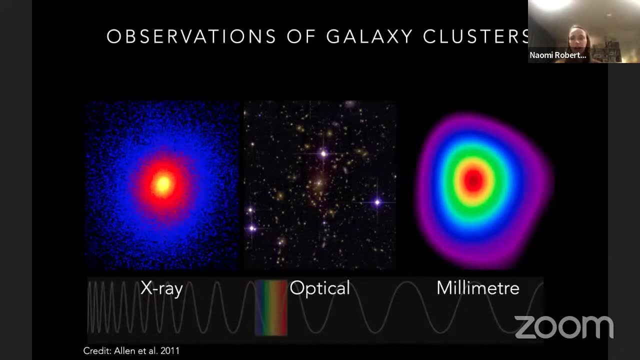 So these are three images here of the same galaxy cluster, but they've been taken with three different types of telescopes. So on the left we see this cluster when we observe it with an X-ray telescope, Then in the middle is the optical. 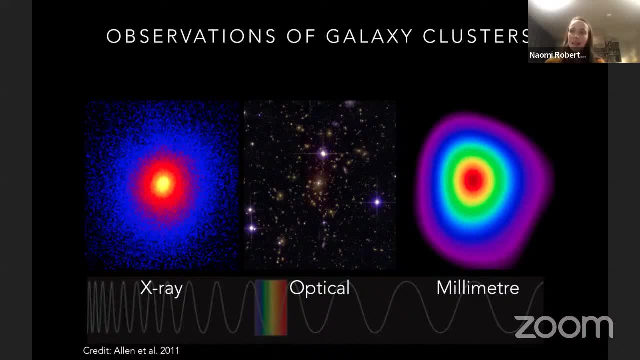 which is similar to the other images I've shown. And then, on the right-hand side, is if we observe the same cluster, but with a millimeter telescope. So galaxy clusters show up in our data across this wide range of wavelengths, which has made them easier to study. 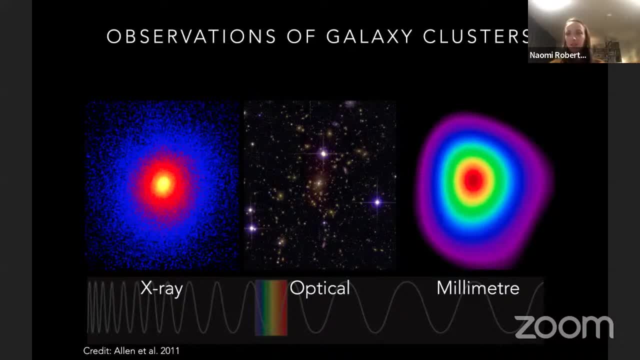 So we see them at short wavelengths with the X-rays, and all the way up to millimeters at much longer wavelengths, And this range of measurements means that what makes up the cluster? sorry, these wavelengths of light include information about the cluster, which in turn tells us a variety of things. 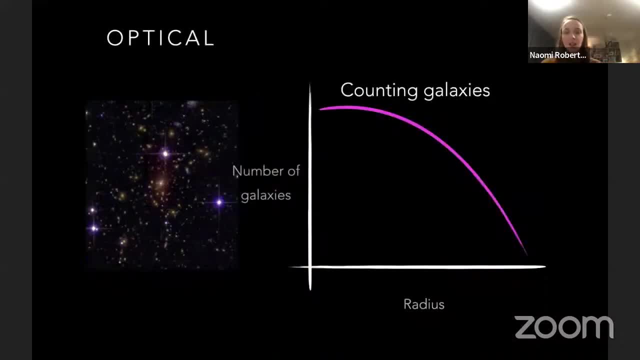 about the clusters themselves. So if we first consider the wavelength that we're most familiar with, which is optical, So yeah, most of the images I've been showing you are optical images, And this is the light that we see with our own eyes. 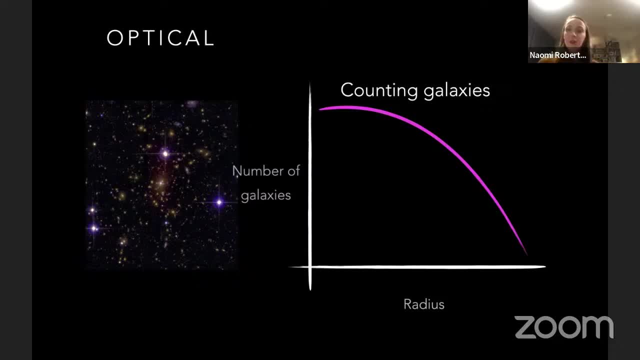 So it was an optical with optical data that clusters were first systematically cataloged back in the 1950s, And the way they were originally found was by looking for over densities of galaxies on photographic plates which were made of the same, So they were called the light of the sky. 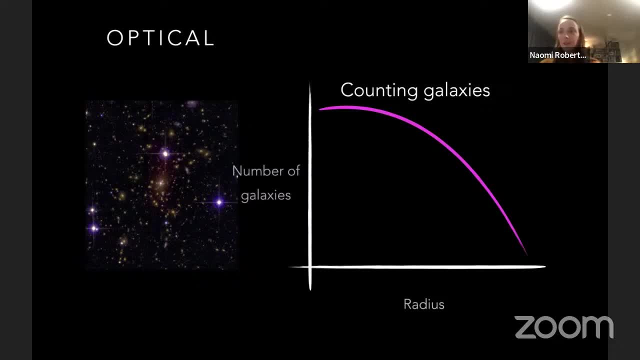 So where do we see more galaxies than anywhere else was essentially the method. So before we had access to computers, this all had to be done by eye. And what astronomers did was they counted the number of galaxies within a certain radius around the bright central galaxy. 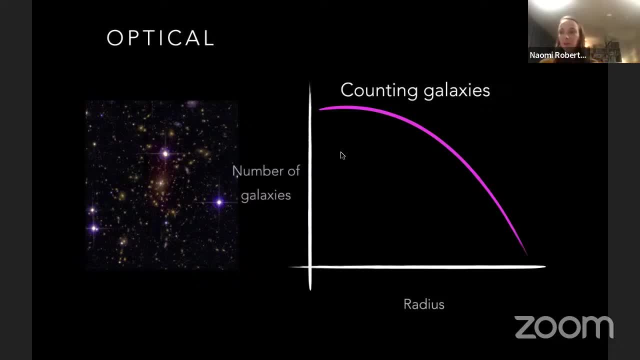 So this is what this plot shows here. So we're towards the center of the cluster, or at small radius There's many, many clusters, And then, as we move out to the edge of the cluster, we find fewer and fewer galaxies. So, using this method, 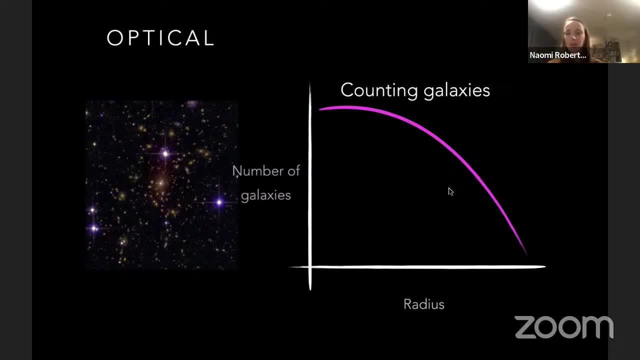 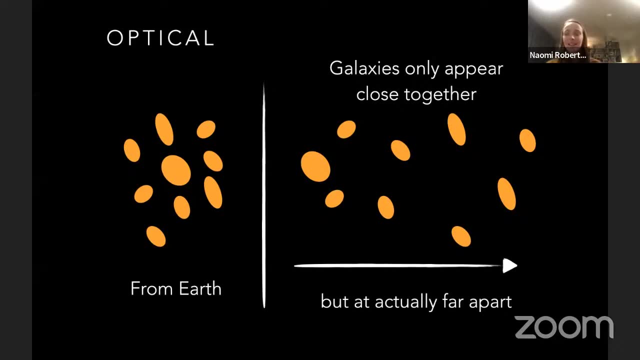 it'd be really easy to find a very rich and bright cluster, and they can be easily identified. The problem with this method, though, is that we could accidentally identify what we think is a cluster, but actually isn't a cluster at all, So this is what's shown here with this toy diagram. 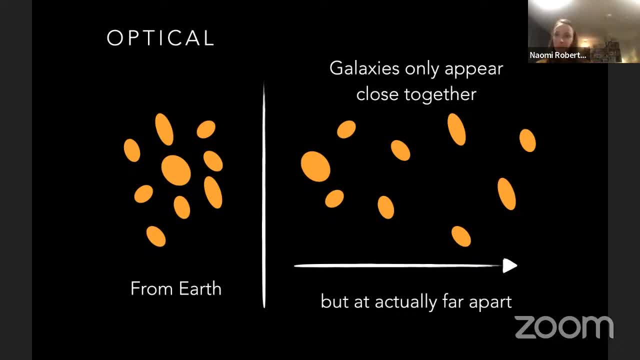 So each ellipse here represents a galaxy. What's shown on the left and the right is what I'm telling you- is the same set of galaxies, but viewed from a slightly different perspective. So from Earth, these galaxies could all appear to be very close together. 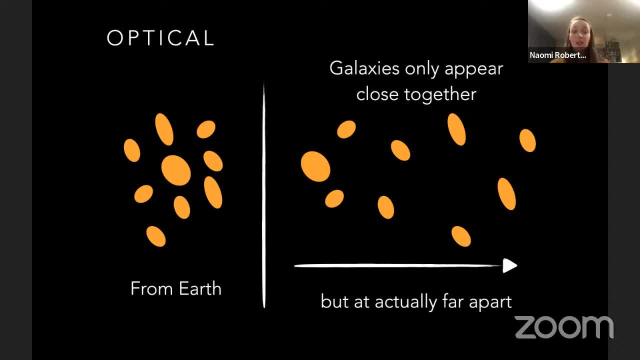 And we could assume then that it is a galaxy cluster. These galaxies may not actually be close together, though, in fact, And when we measure the distances to these galaxies, we find that they're actually separated quite significantly, And they just appear to be very close together. 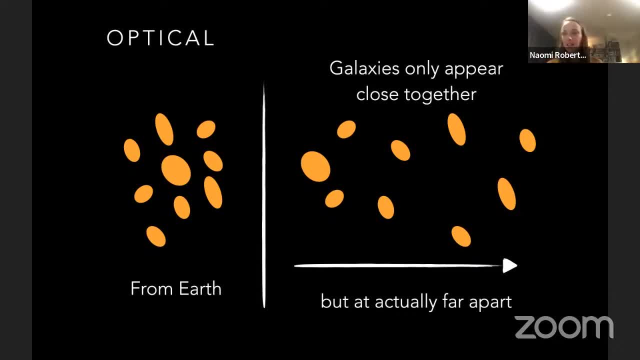 And they're not necessarily aligned by chance, And this is what's shown on the right hand side. So if we could look at the galaxies from a slightly different angle, we'd know this. So the way we can avoid this and check that we haven't misidentified any of these clusters- 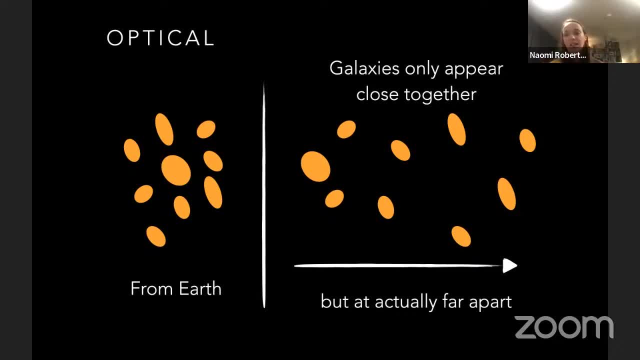 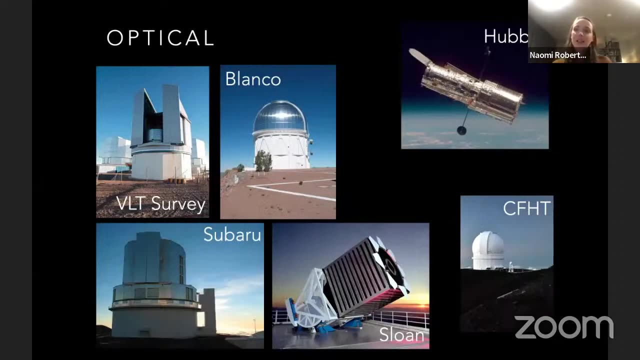 is by ensuring that we have really good measurements of the distances to the galaxies. And measuring to the distances to galaxies in a cluster becomes more and more difficult when the cluster is further away and therefore fainter. So some of the telescopes that have been adding to this now huge catalogue of clusters 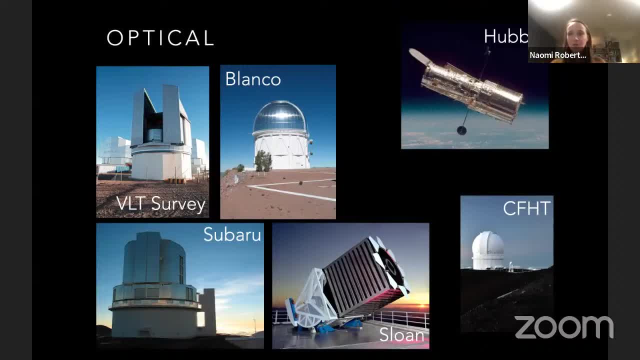 are shown here, And these are the telescopes which are responsible for those really beautiful cluster images that I showed earlier, And we keep continuing to build up these catalogues with even better data as well. So these telescopes are at many different locations around the world. And we also have the Hubble Space Telescope, which is actually up in space, And many of them are located in Hawaii and Chile, as these are the best observing sites, as the atmosphere is a lot clearer, So it's the closest we can get to space. without actually going to space, And having a telescope on Earth is actually a benefit. as we get a bigger, we have a bigger telescope mirror and therefore look at a much wider area of sky, And it's also a lot easier to fix if anything stops working. 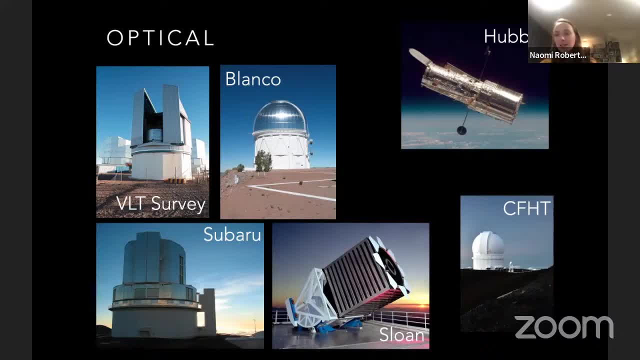 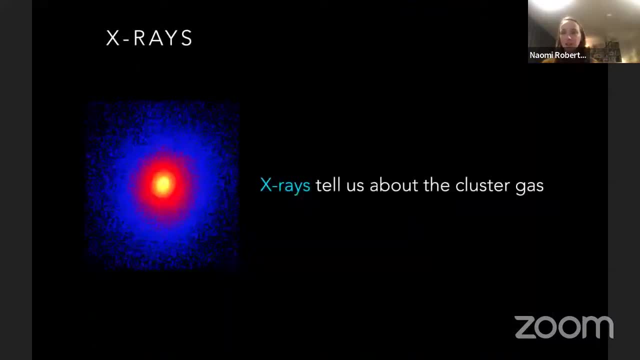 Looking to the future, there's also more optical telescopes planned and currently being built which will add to these observations. So now, moving on to our second method, our third method of detection. We can see galaxy clusters with X-rays because the gas in the cluster falls in towards the centre. 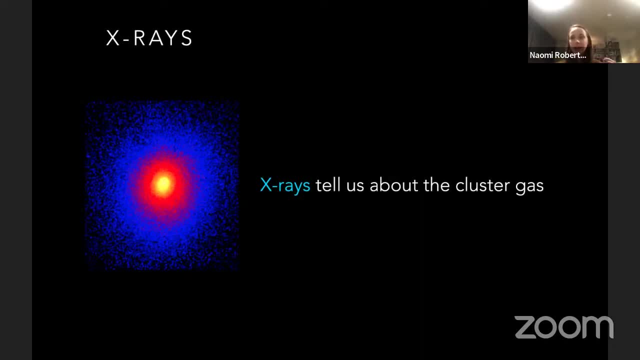 due to the gravitational pull of the cluster itself. So the gas gathers speed as it moves towards the centre And at some point the particles of gas will collide and then this emits X-rays, which is what we see here. So the centre of the cluster is brighter. 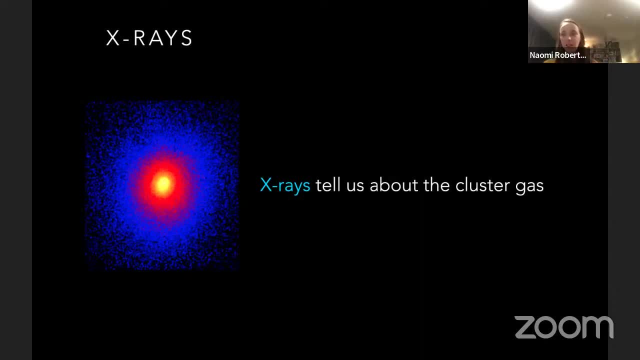 compared to the outer regions. when we look at the X-ray data, So looking at a cluster with an X-ray telescope, they appear very clearly in our data, but these observations we no longer see the individual galaxies inside the cluster as we did in the optical data. 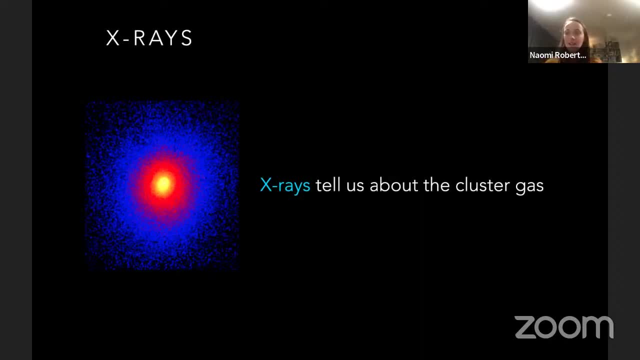 And instead. this is because the hot gas inside the cluster lives in between the galaxies, which is what we call the intracluster medium, And this is concentrated. well, it gets more and more concentrated towards the centre, So this hot gas is diffuse. 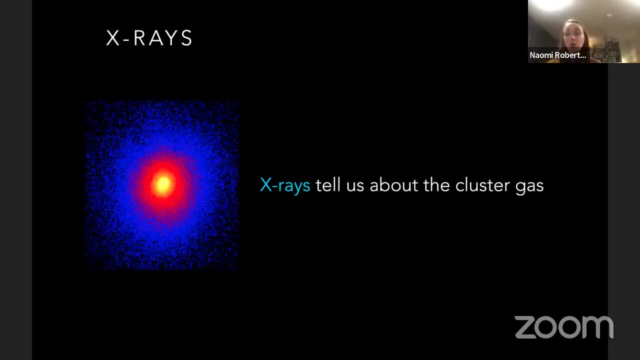 and the space between the galaxies. and using these X-ray observations we find that there is, on average, about seven times more mass in the hot gas than if we were to add up all the stars and all the galaxies that live in the cluster together. So by measuring how bright the X-ray signal is, 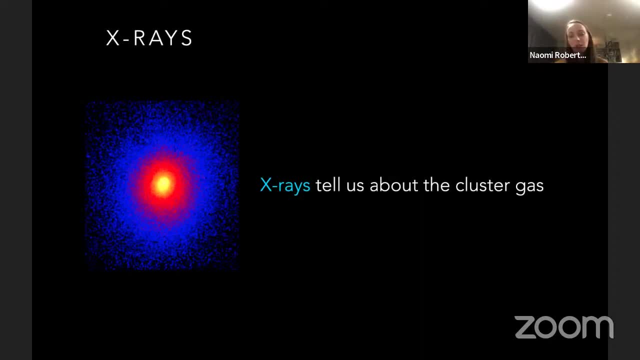 or the X-ray luminosity, we can get information about the gas inside the cluster. So X-ray luminosity tells us how hot and dense the gas is inside the cluster, which is why the colour of this image on the left hand side changes from being yellow in the centre. 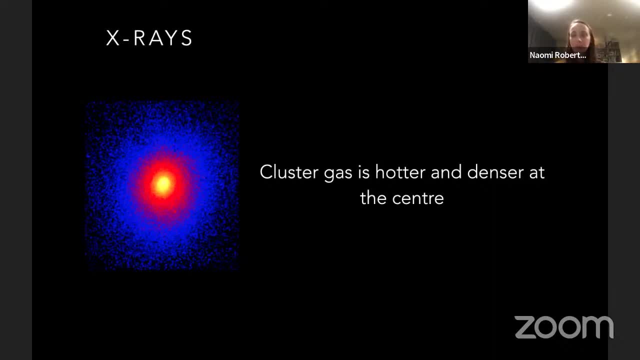 where it's very hot and dense, to being blue on the outside, where it's slightly cooler and less dense. Now, the reason the gas is hotter and denser in the centre is because the pressure on the gas due to gravity is strongest there, So we can therefore use these measurements of gas pressure. 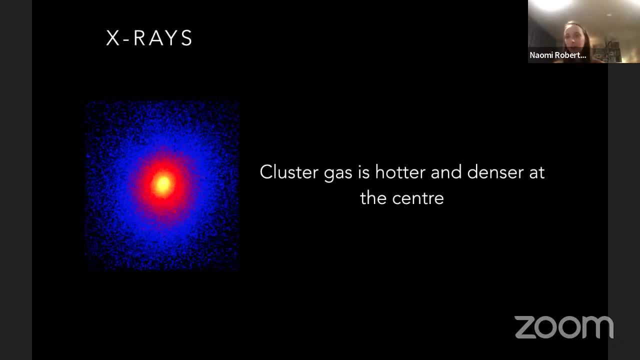 to infer how much mass is in the cluster. And this is one of the ways that we know that clusters contain so much dark matter, as by counting off all the galaxies and measuring where the mass content is, we see how much that weighs, and then we can compare that to the mass that we need. 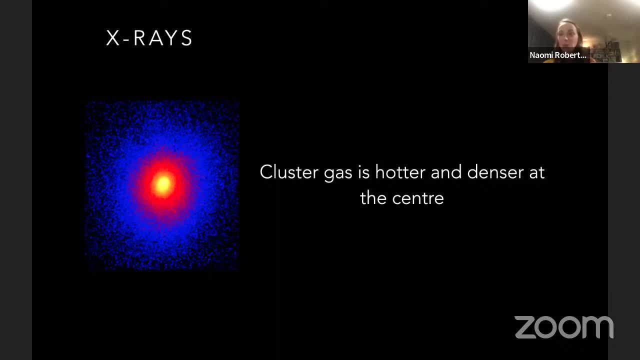 to hold the cluster together, And what we find is that we actually need more mass than we see, And this is one of the ways in which we've inferred the existence of dark matter in galaxy clusters. So this is an indirect way and it depends on how well we understand. 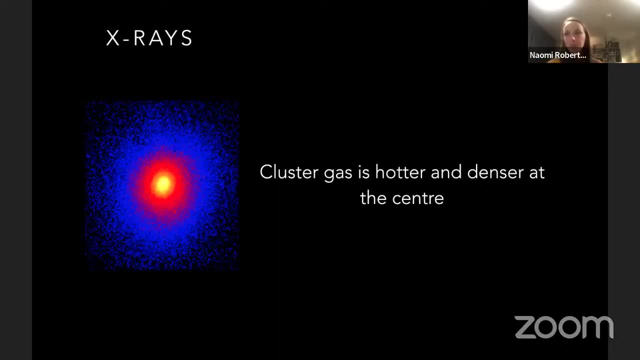 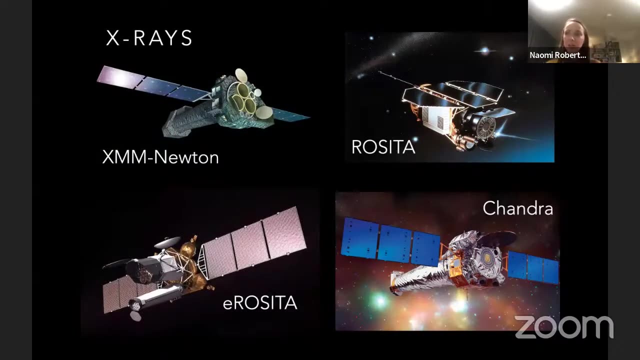 the physics of the gas inside the cluster. So we can't make observations of X-rays from ground-based telescopes because X-rays are actually blocked by Earth's atmosphere. So here are the main X-ray telescopes, So you can see they're all space telescopes. 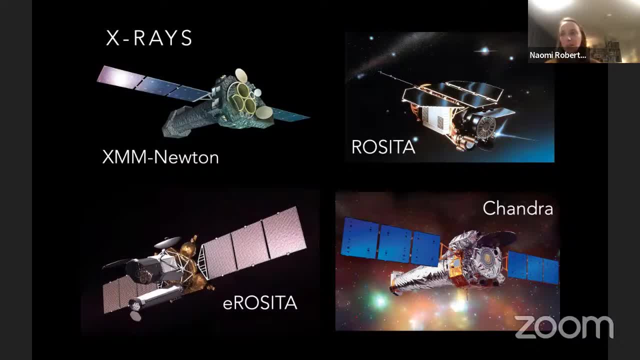 which have contributed to the X-ray cluster samples. So E Rosetta, which is shown in the bottom left here. this is the newest telescope in the fleet of X-ray telescopes looking at clusters, And this is what the sky looks like to E Rosetta. 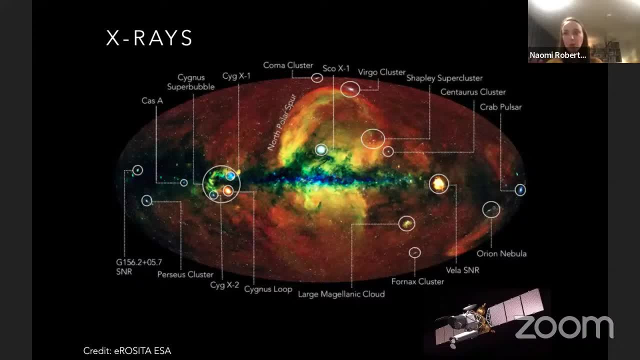 So E Rosetta observes the whole sky and detects any X-rays that have been emitted. So our own galaxy emits X-rays and we see that across the middle of the image And we can also see, for example, the Virgo cluster. 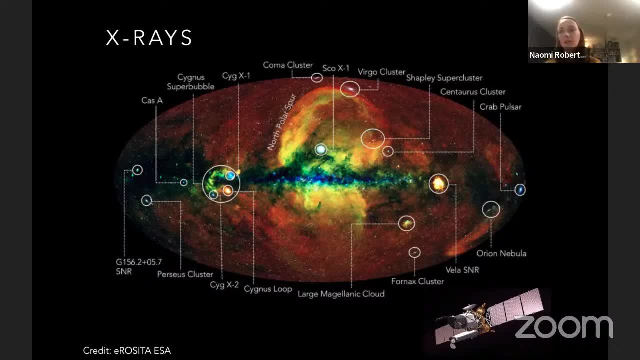 which I showed you earlier. at the top of this image And some other nearby clusters are also clearly visible, And many of the other bright objects that we see here are other objects either in our outer galaxy that also emit X-rays. So now I'm moving on to our final method for finding clusters. 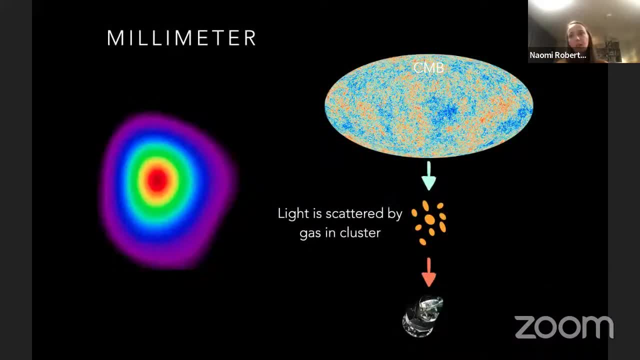 which is with millimeter telescopes. So when we look at the sky with a millimeter telescope, we see radiation coming from all directions And this is what we refer to as the cosmic microwave background. So the cosmic microwave background, or the CMB, 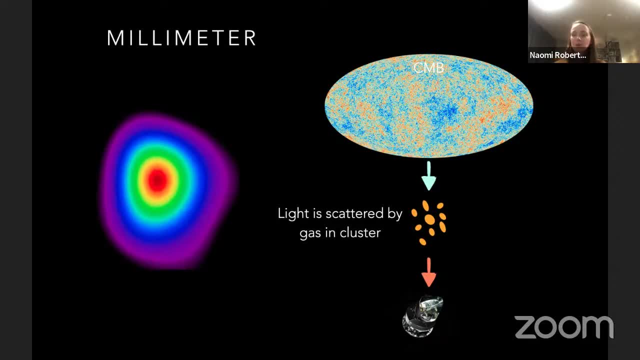 which is shown at the top right. here is light left over from an early stage in the history of the universe. This is actually the oldest light that we can see, As this ancient light travels through space en route to our telescopes here on Earth. 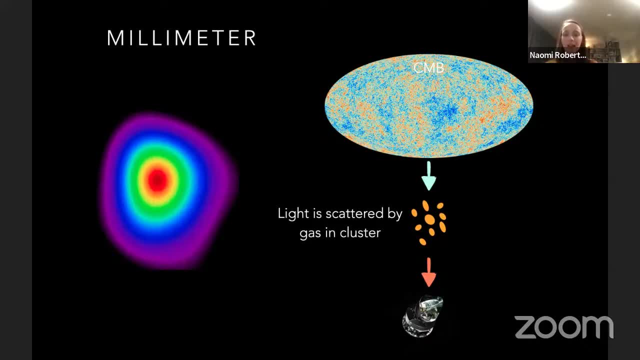 if this light encounters a cluster, it can be scattered by the hot gas that's inside the cluster. So as the light passes through the cluster it's slightly changed as it interacts with that intracluster medium. So when we make measurements of the cosmic microwave background, 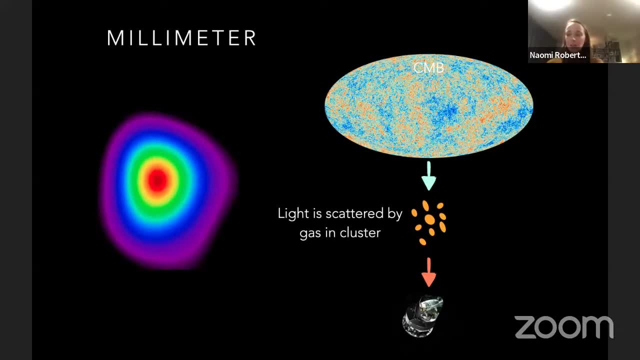 with our own telescopes. the clusters leave their marks on the data, almost like a fingerprint, And this fingerprint only helps us find the galaxy clusters in the data. It also contains information about the gas inside the cluster as well. So because the cosmic microwave background has traveled such huge distances, 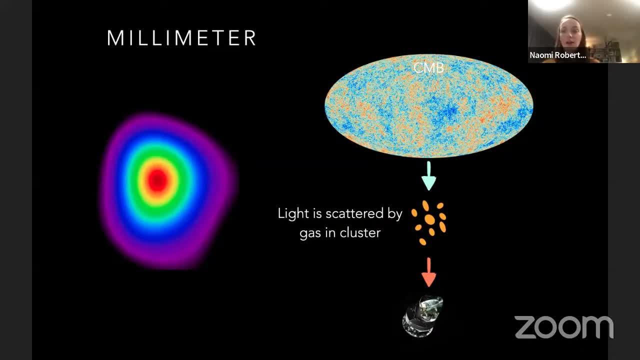 it means it can be used to find clusters that are really far away And, as we know, when we look further away we're looking further back in time to when the universe was younger. So with this method we can see clusters early on in their evolution. 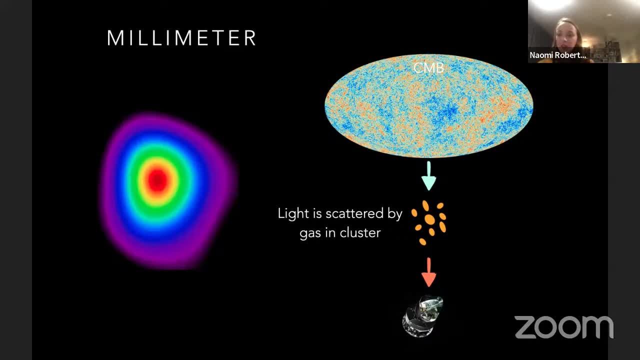 Since it's a very complex system. we can use the gas in the cluster that causes this effect. We can use these measurements to learn about the gas properties in a similar way to how we did with the X-ray data. And again, this is another way in which we can infer. 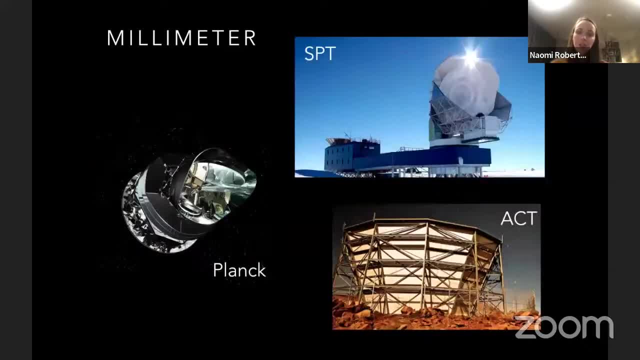 how much mass is contained within the cluster itself. So in the last few years we've seen a huge increase in the number of clusters that have been detected using millimeter telescopes, And this has been primarily from these three telescopes shown here. 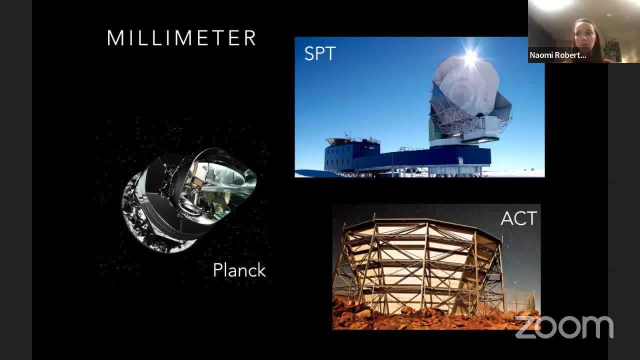 So Planck is shown on the left-hand side. This is a space telescope And this telescope found around 2,000 clusters using this technique. We also have the South Pole Telescope and the Atacama Cosmology Telescope, And you can take a good guess of where those telescopes are located. 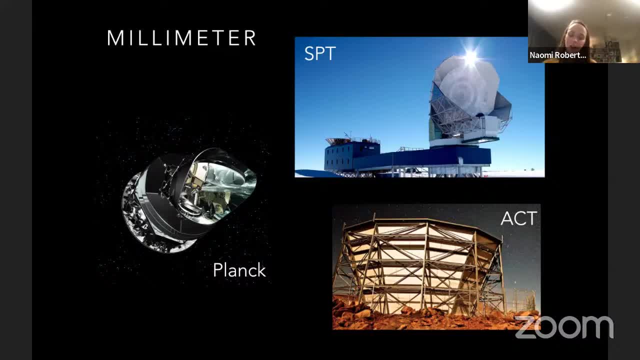 And because these telescopes are ground-based, they can have much bigger mirrors because we don't have to pump them up into space, And so because they have bigger mirrors, they have better resolution. So we therefore have better tools to be able to detect these clusters. 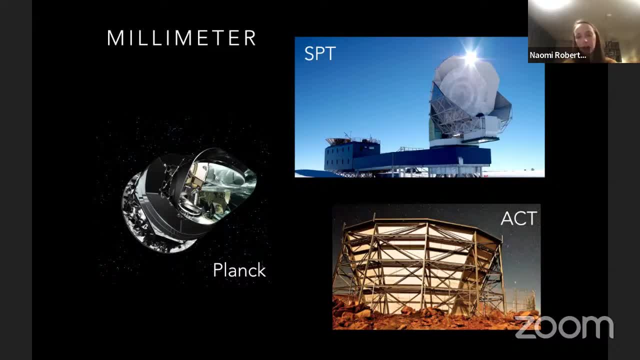 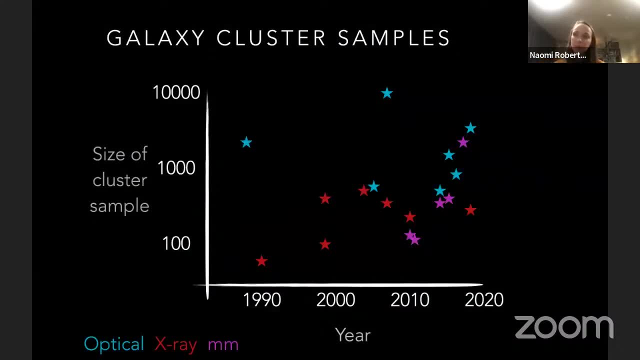 Even more clearly and find clusters that are actually even smaller. So with these three methods we've now accumulated a huge sample of clusters, And this plot here shows how many clusters were detected at different years over the past 30 years or so. 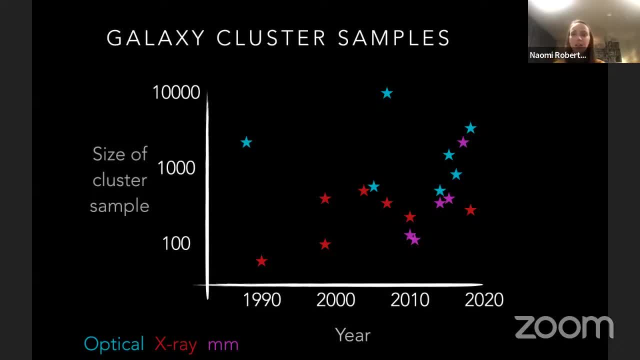 So each star on this plot corresponds to a different data set And the color corresponds to which type of telescopes being used. So blue is for optical and the red for X-ray and then the purple for the millimeter telescopes. So looking at how these cluster samples have increased over the years, 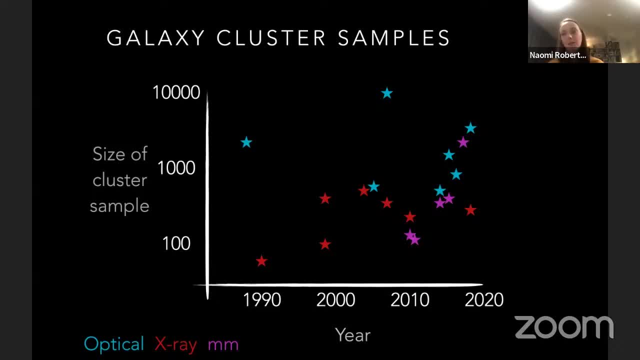 we now have samples of around 5,000 from both optical and millimeter observations, And the X-ray data is nearly up to 1,000 as well. So we've really ramped up our sample size, And the aim is to be able to observe as many clusters as we can. 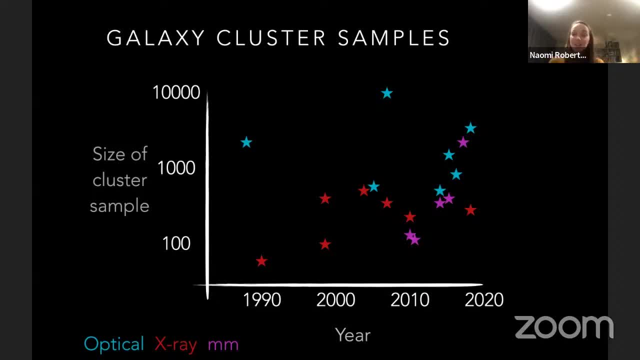 in the observable universe, And there are many different reasons to study galaxy clusters. They're really interesting just to look at how the galaxies live inside these really dense environments, But why I'm interested in them is that they can tell us about how our universe came to be and the structure in it. 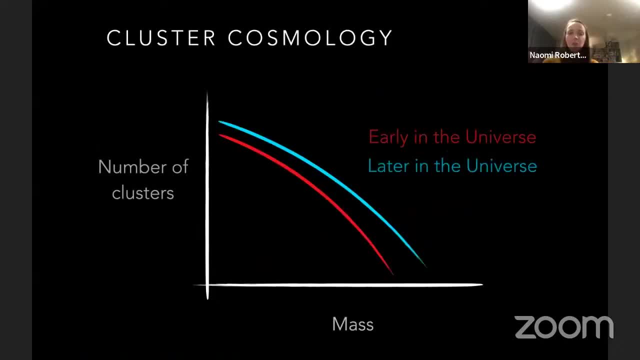 and how that formed. So, with observational methods I have been describing, what we're trying to do is understand how many clusters we see at different times in the history of the universe, and how big these clusters are. So then, from our best theories of cosmology, 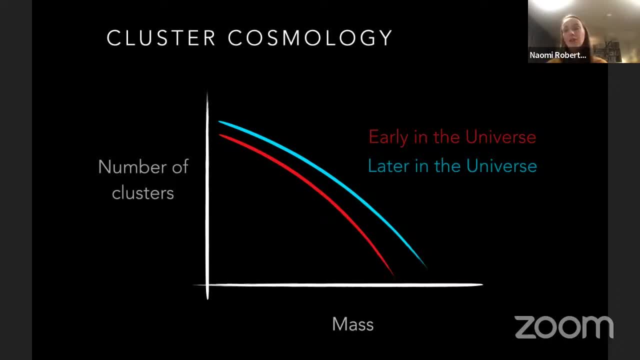 we have an idea about at what point we should see the first clusters emerge, And by looking at how big they are, we can also understand how they've grown and evolved over time. So this can help us understand that matter, since clusters contain so much of it. 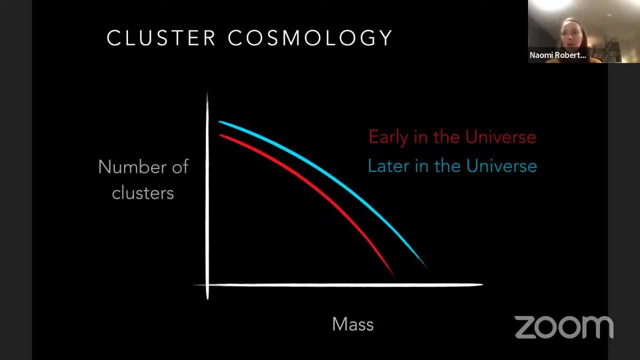 For example, if clusters are more compact than we expect, or they grow bigger and much quicker than we expected, then this will tell us we need to update our theories of how the universe works, And so what I've plotted here is just really, we're trying to find the number of clusters. 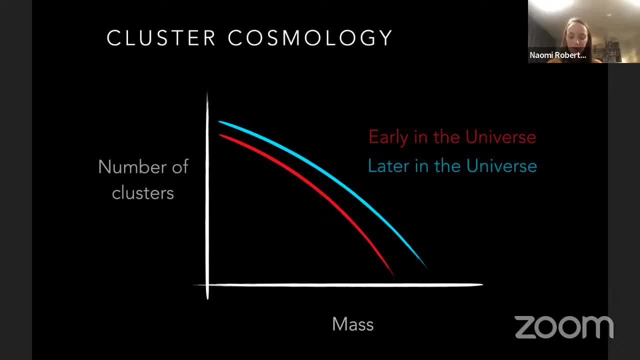 for a given size of cluster and try and map this out at different points in the universe's history. Now, we can't see dark matter directly. However, we can find out where it is and how much is there another way, And this is using a technique called gravitational lensing. 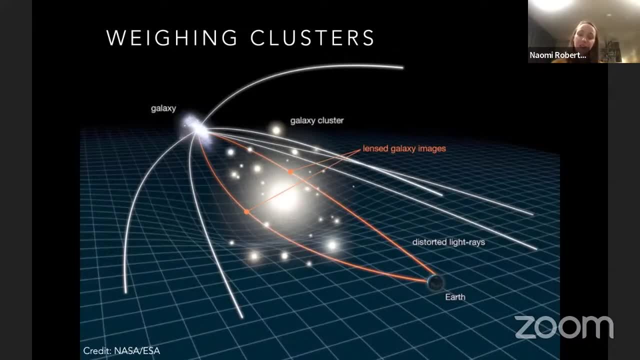 So gravitational lensing is based on Einstein's theory of relativity, which said that the fabric of space-time itself is bent by the stuff that inhabits the space, And this is what is represented here. So, with the space represented by a grid, 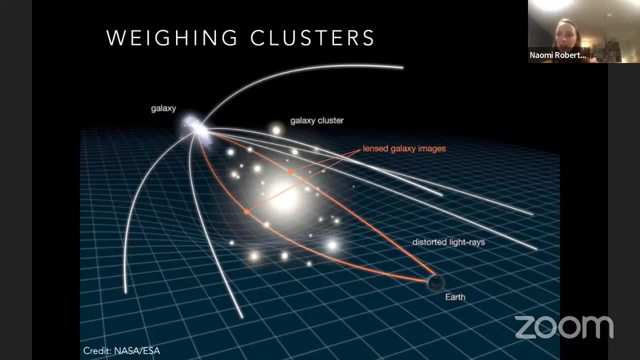 and then we have a galaxy cluster in the centre and a galaxy behind this cluster. So here on Earth, which is down here in the bottom right of this diagram, we're trying to observe that background cluster. So if this galaxy cluster wasn't present, 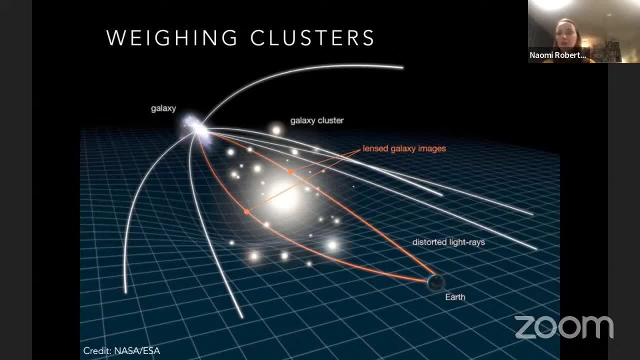 then the grid would just look flat and so the light would travel straight towards us. But if we put the cluster in between us and the more distant galaxy, we find that it distorts space, and then the light from that background galaxy doesn't travel in a straight line anymore. 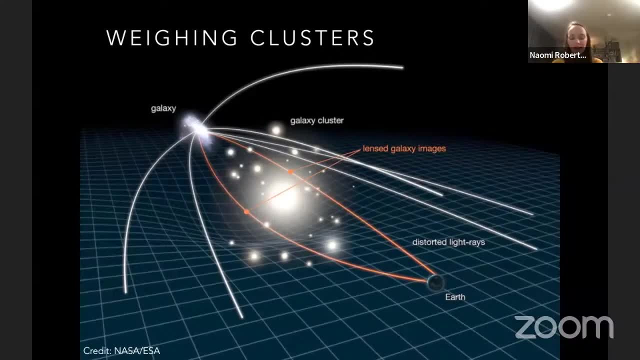 It's distorted and takes a different path, And so the way I like to think about it is: if you imagine a mattress and you were to just roll a marble across the mattress, it would just follow a straight line. However, if you were then to put a heavy weight on the mattress, 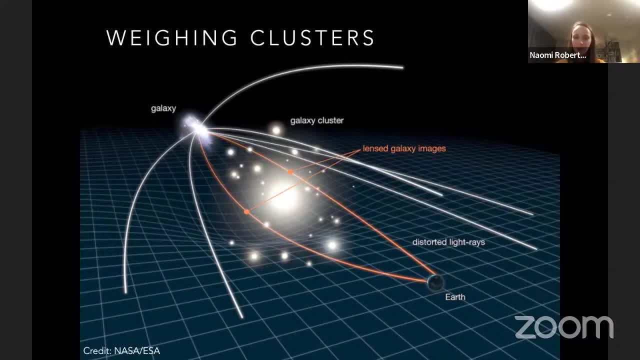 like a big bowling ball or something and try to roll the marble kind of close to where the bowling ball was. it would no longer follow the straight line because the shape of the mattress has been changed by the bowling ball. The marble would follow a slightly different path. 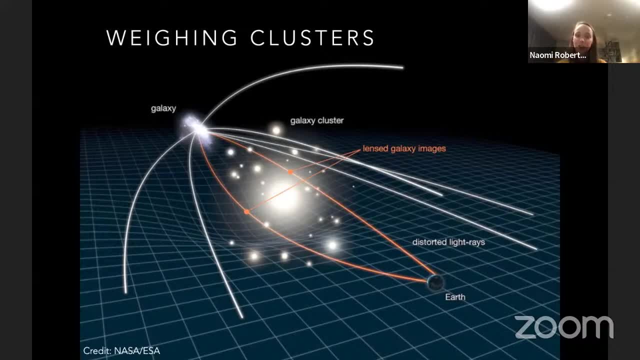 And this is exactly what happens to light in our universe as it passes by these huge galaxy clusters. So if we can measure this change or this distortion in the light from distant galaxies, we can find out about the mass that is causing the distortion, which, in our case, is the dark matter inside these galaxy clusters. 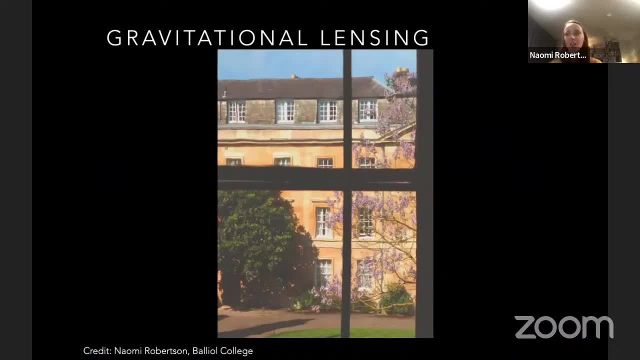 And so this is similar to looking through a magnifying glass, where the thickness of the glass varies around the lens, across the lens, sorry. So here we're looking through a magnifying glass, through an old window, And if we zoom in on these two windows, 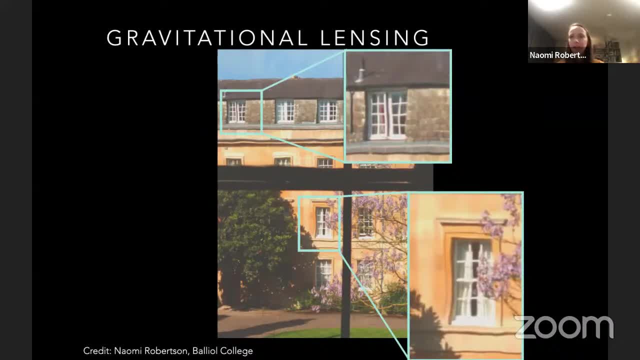 we can see that things don't look quite right. So the thickness of the glass- because it is one of these old-fashioned windows- is different in different places, And so our image of the outside world appears distorted, And this is what is happening with galaxy clusters. 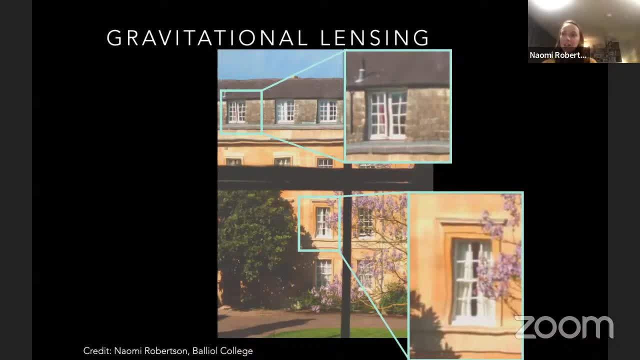 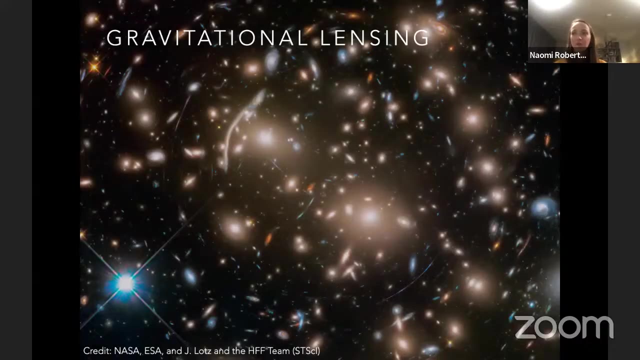 but instead of it being the thickness of the glass that's changing, it's actually how much dark matter is present in our cluster changes, And this is what we see in data, Especially in the most massive clusters So like this one. So if we look at this image for just a few seconds, 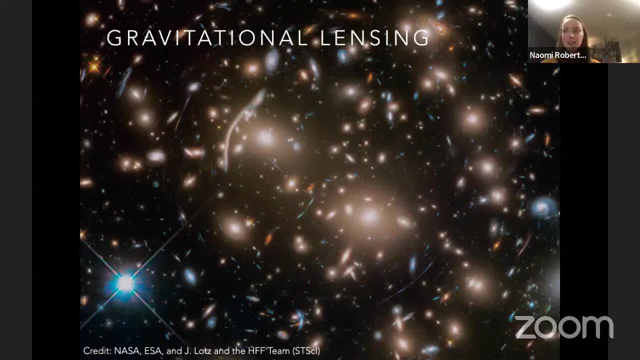 can you see the distorted light or the gravitational lensing of the background galaxies, And can you see where the galaxy cluster is here that's causing this effect? So we see the cluster in the centre here, and these giant arcs around the outside are, in fact, light from more distant places. 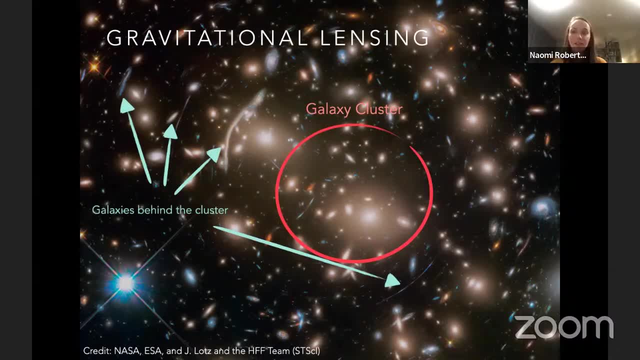 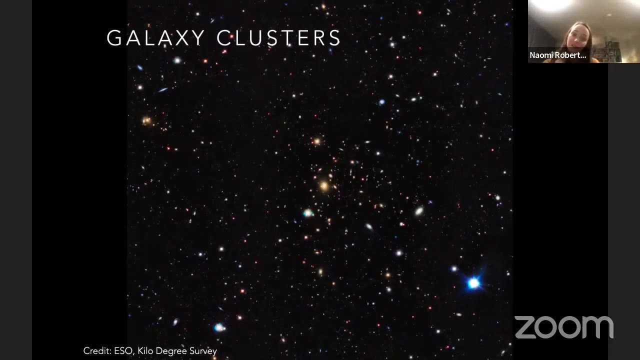 So we can see that these distant galaxies that have been stretched because of this lensing effect, And so by measuring how distorted these distant galaxies appear, we can reveal where the dark matter is. So this is an image of a galaxy cluster taken by the kilodegree survey. 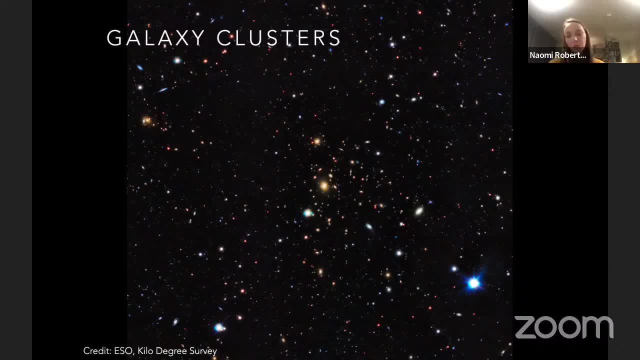 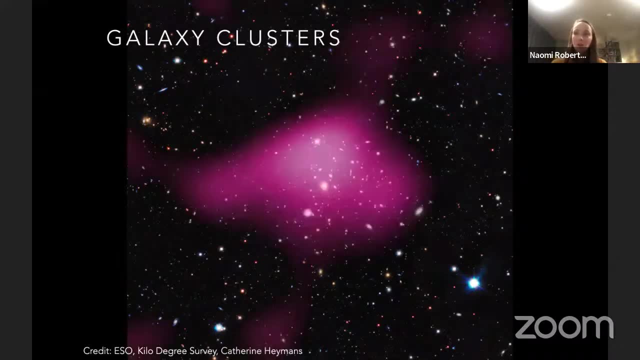 And part of the aim of the kilodegree survey was also to measure this gravitational lensing effect. So if we take the gravitational lensing information, we can map out where the dark matter is, and that's what's shown by this pink fuzzy blob here. 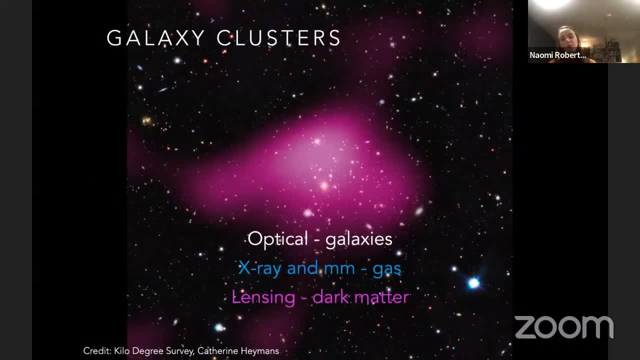 And so, by using all these observations together, we can learn about the different components of galaxy clusters and how they have formed and evolved, And so this is the work that I'm involved in. So, with the Atacama Cosmology Telescope, this observes a millimetre light. 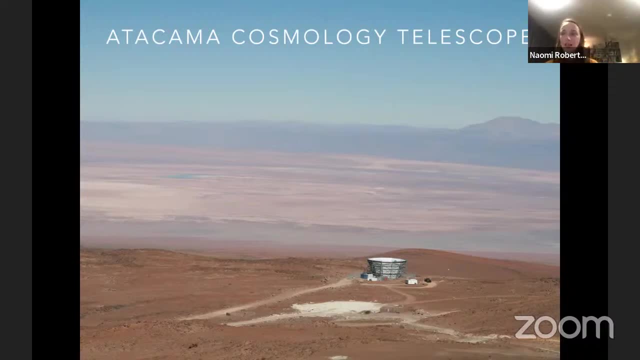 and we can use this telescope to detect where galaxy clusters are. So this telescope is located in Northern Ireland, Northern Chile, so it sees most of the southern sky And these observations tell us where clusters are. And this telescope has really great resolution and has been used to find even smaller clusters. as a result, 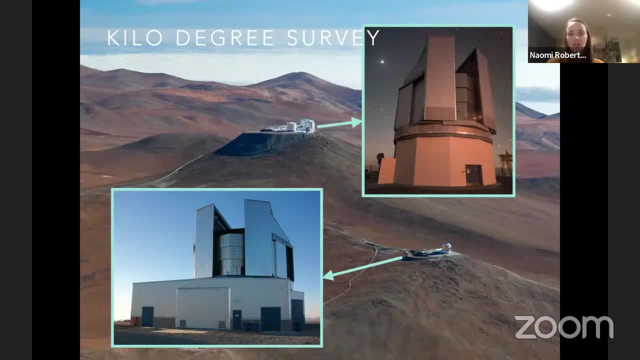 We can then use our observation from these two telescopes- So this is the VLT survey telescope and the VISTA telescope, which are both located at the Paranal site, also in Northern Chile, And this is what forms the kilodegree survey. 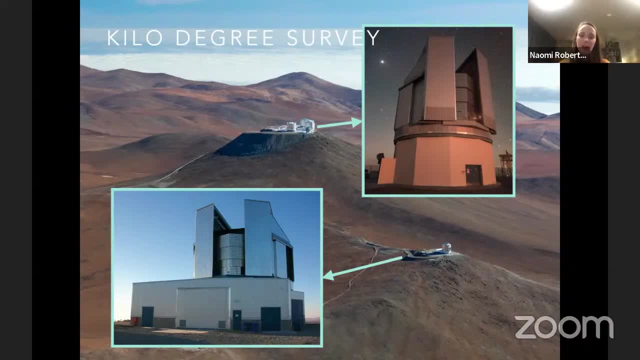 And because these telescopes observe the same patch of sky as the Atacama Cosmology Telescope, we can make gravitational lensing measurements around the clusters that the Atacama Cosmology Telescope has found, And that's what we've done with around 200 galaxy clusters. 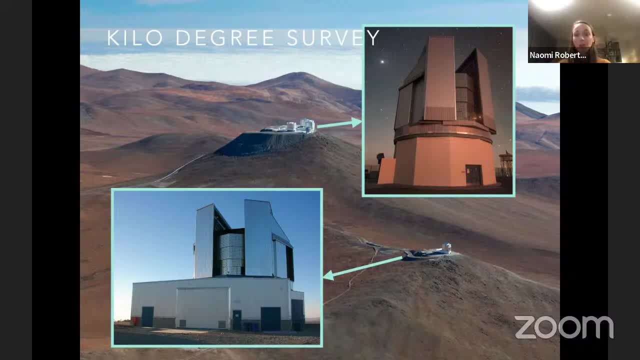 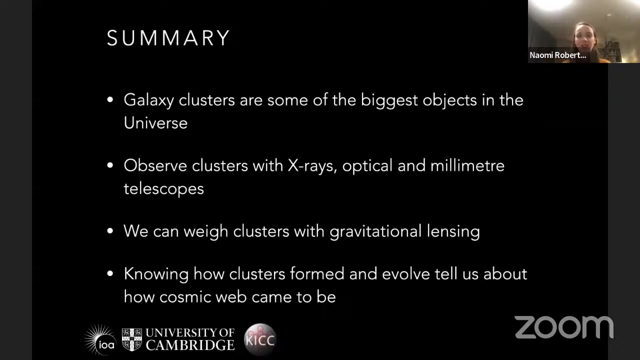 We've been able to measure their masses And we're using these measurements of their mass and their gas to try and understand cosmology better with these results. So I'll just summarise what I've told you here about galaxy clusters this evening. So these beautiful giants are really quite incredible. 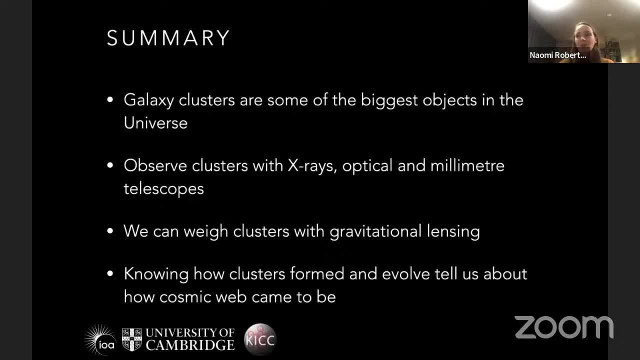 and they literally are more than what meets the eye. Through observations of X-ray, optical and millimetre telescopes, we've been able to understand them much more deeply and, more importantly, the seemingly invisible dark matter which is such a huge part of our universe. 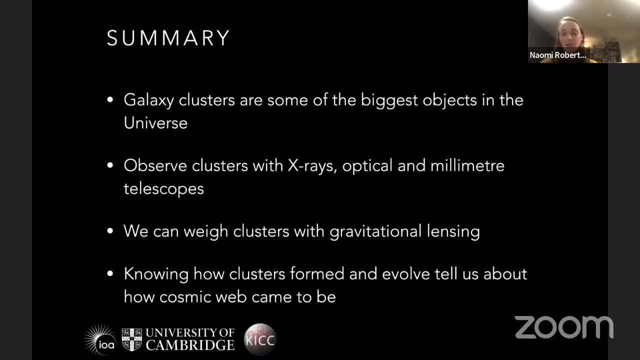 These clusters hold information that we need to understand how the universe came to be, which is one of the reasons why we're so interested in studying them. So thank you for listening, and I'd be happy to hear any questions you may have. Wonderful Thank you so much. 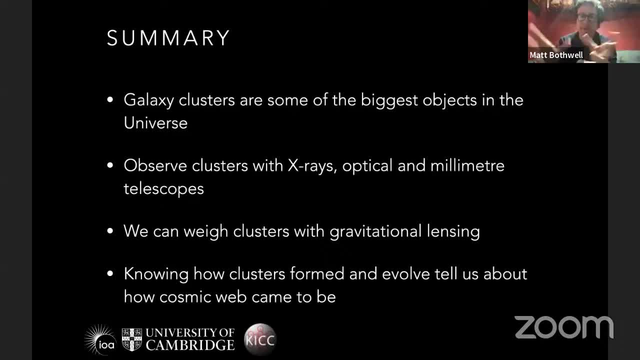 It's so fascinating. I love seeing those wide field images with all those lensing arcs around the clusters. They're always so striking. If you have any questions for our speaker, please pop them down there in the YouTube chat box. On a kickoff, I was asking you something. 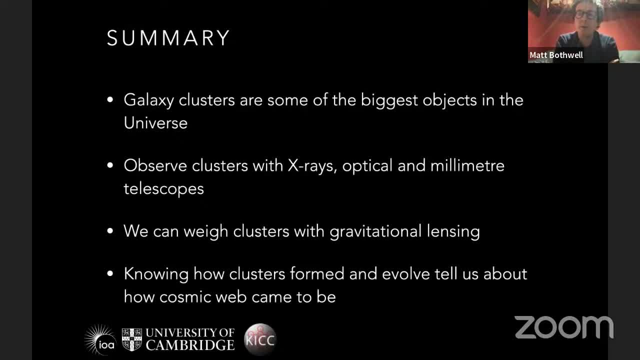 that I was thinking about as we were going along, Because VBs are such a fascinating subject. What are some things that we don't know about clusters? What are some of the open questions in galaxy cluster research that maybe you're working on right now? 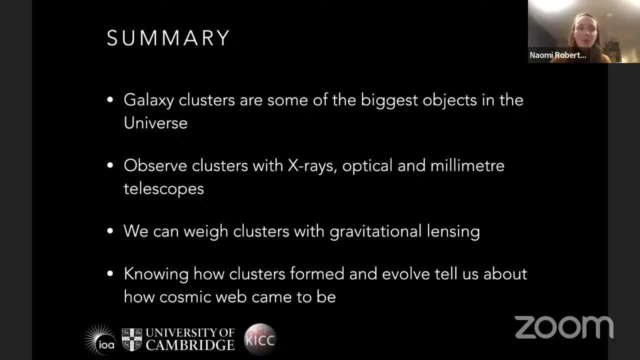 or maybe something that you'd love to know? the answer to Yeah. so one of the things that is most challenging, which has really been the sticking point in being able to do cosmology with clusters, is trying to really pin down this mass. 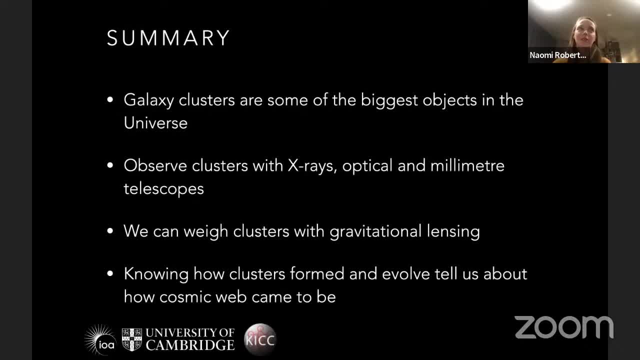 So I've made it sound really easy here that we just do gravitational lensing and then the mass pops out. But in practice that is complicated by things like the gas and the clusters themselves. So we're only just starting to understand or even investigate how these two things interact. 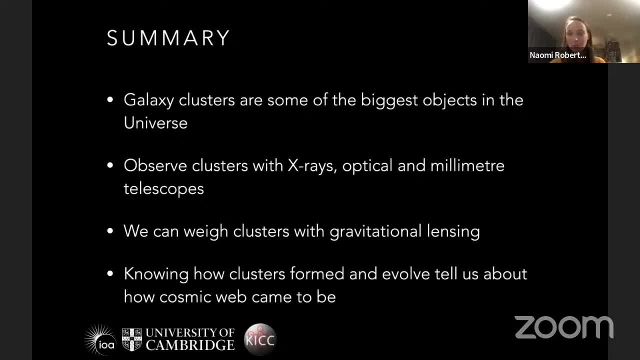 and how the gas and the cluster actually affects the lensing measurements, Because when the gas moves around, this changes the lensing measurements themselves, And we've kind of ignored that till now. So what I really want to understand is the connection between those two things. 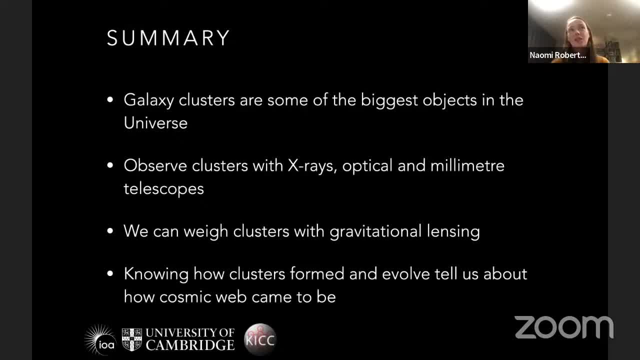 And also things like: when we make these measurements, we assume that galaxy clusters are perfect because they're perfect spheres and they all stick quite nicely, Whereas in practice we know that that's not the case at all. So I think what would be really interesting again, 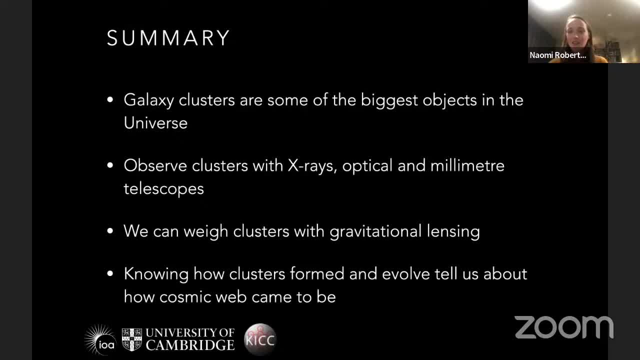 is to see, with simulations, whether they can predict what happens when, say, galaxy clusters undergo mergers, Because they're not just balls of dark matter sitting out there in the universe, They're really active and the galaxies inside them interact and they eat other clusters that come past and stuff like that. 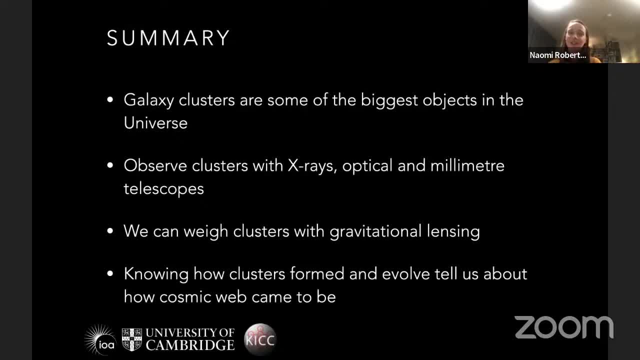 So there's a lot going on there. So it's trying to understand how the dynamical part of the galaxy clusters actually impact these mass measurements and then how this changes our cosmology. Amazing, It's fascinating stuff. There's a question. come in from Julian on the chat. 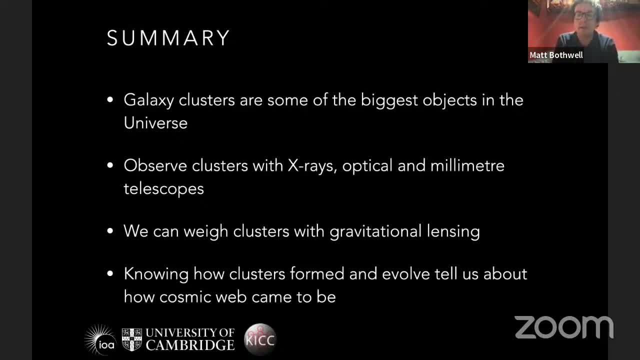 who wants to know? do we have a good sort of mathematical understanding of how clusters and filaments and voids form in the first place And are the formation of these things? can we reproduce that with models? Can, yeah, to a degree. yeah, we definitely can. 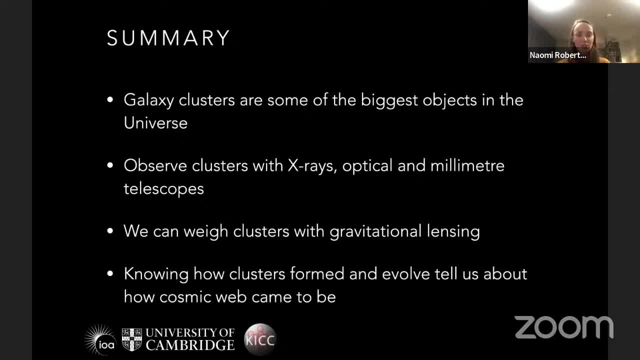 So we think that there was these tiny fluctuations in the early universe that really sparked off where the positions of these clusters then came to be, And that we think that the matter grew by this hierarchical merging. So you had one small fluctuation and then, because of the way gravity works, 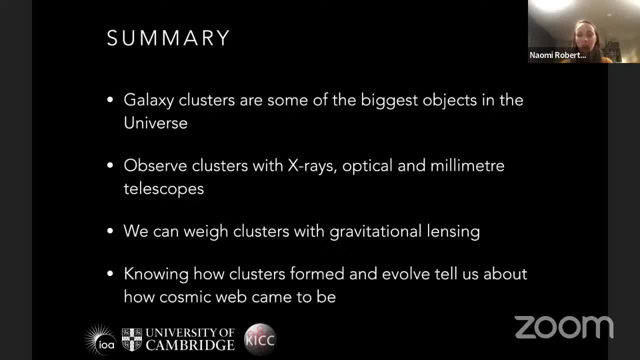 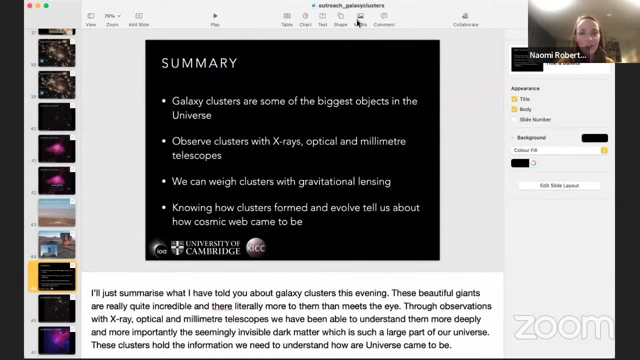 it just pulled in more and more material And so over time I think I actually might even have to go back to that. Oh no, I don't, Nevermind, I'll go back to that. I thought I had a video actually that showed this. 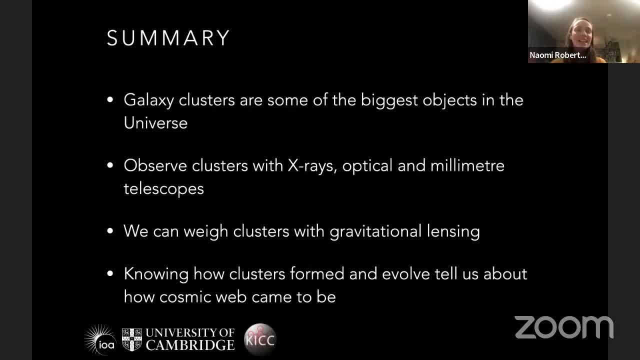 in my backup slides. But yeah, so it pulls in more and more material over time And if we run that through we're just with our kind of ingredients for how we think that the universe came to be. we see these filaments exist. 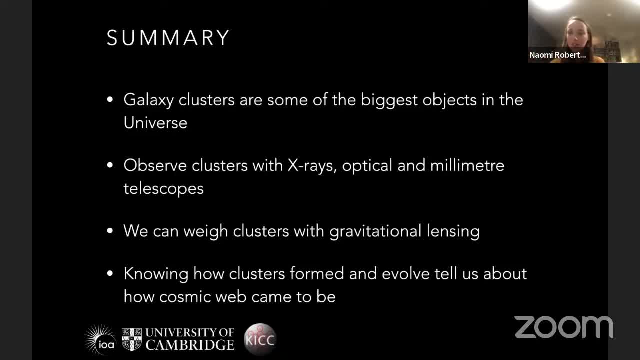 come into existence just by this process of gravitational collapse to form the clusters, The real now. we're now getting into kind of like the nitty gritty of this And what we're trying to ask is: are the clusters as big as we expect them to be? 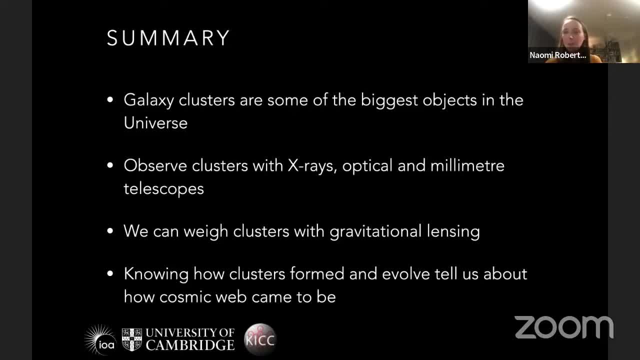 Are they? should they be smoother or should they be clumpier? And but we think we have a good idea of actually how the structure itself was formed through this process of gravitational collapse and merging and so on. Excellent thanks. There's a question from Karen. 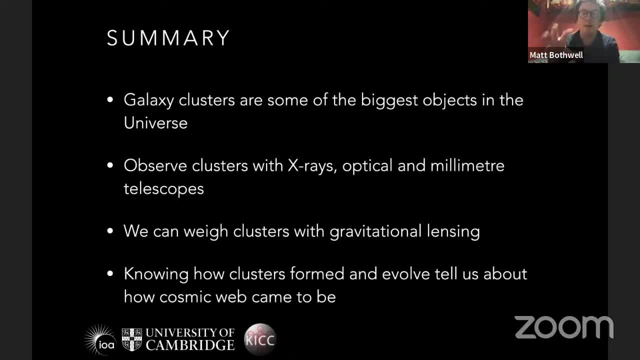 I think could you describe a little bit more about how clusters can curve space and cause this gravitational lensing effect? Because the question is sort of: you showed this picture of a dent in space And I'm just wondering that wouldn't you also get a dent in space? 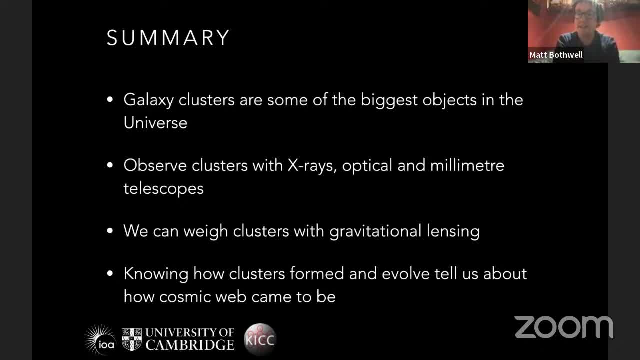 sort of above the cluster, and those two things would sort of cancel out. Maybe if you could just describe how it sort of works in 3D a little bit, Yeah, it's really hard to actually try and get a good image of what's happening. 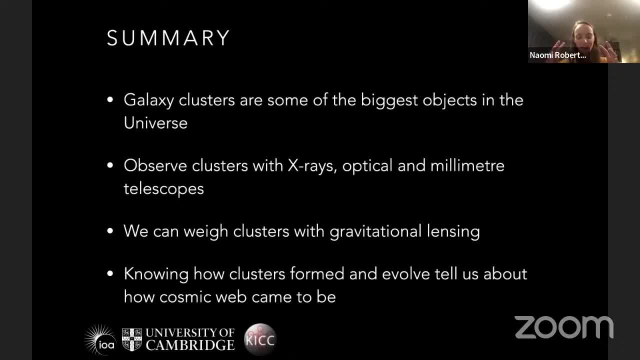 because we're limited to a 2D screen as well. So, yeah, so the cluster will destroy the whole of space in these three dimensions. So what happens is, as light comes past, instead of it travels as a straight line through 3D space. 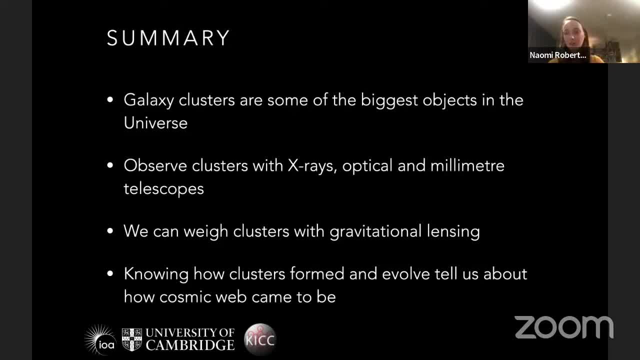 but it can either be distorted up the way or down the way, depending on whichever path. So it'll just: the path will only be switched in one direction. Hopefully that makes it a bit clearer And what we actually see with these giant arcs. 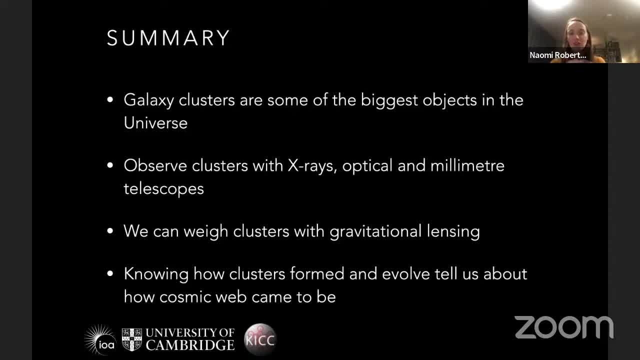 and stuff is a galaxy isn't just a single point source of light. It's actually got many photons of light emitted from that more distant galaxy. So what can happen is one bit of that galaxy. the light from that galaxy will be distorted up in one direction. 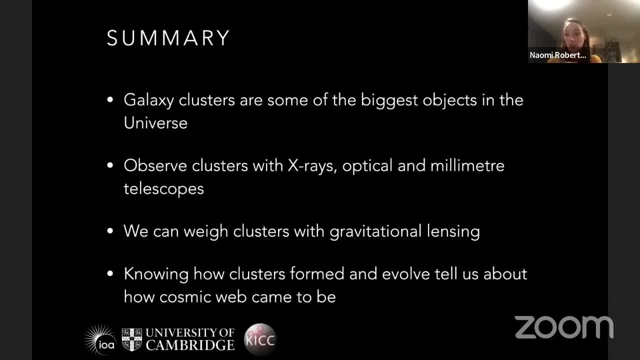 And then as you move along, because the distortion of the space-time has changed slightly, light emitted from another part of the galaxy will be distorted in a slightly different way, And that's how we get this stretching is because different parts of the galaxy are different parts of light. 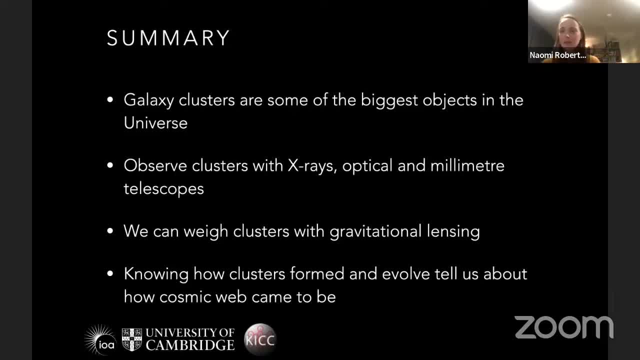 and they will take different paths. Maybe that was more confusing, actually, And I think that's a good explanation. I think it's always. I think it's fundamentally because you know we can understand a 2D space. you know a 2D sheet being curved or something.